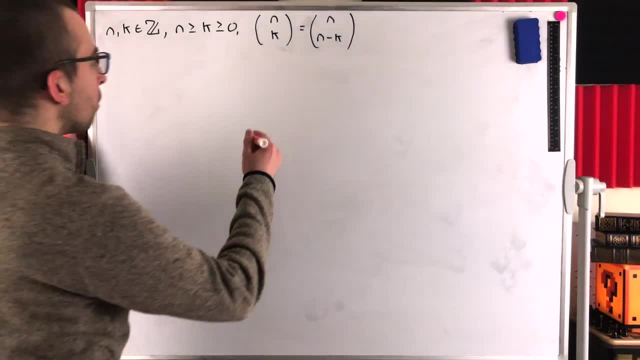 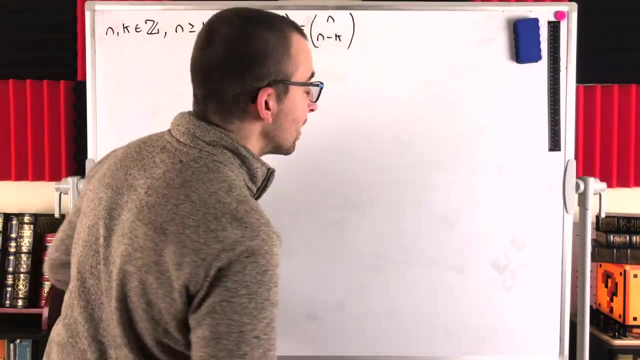 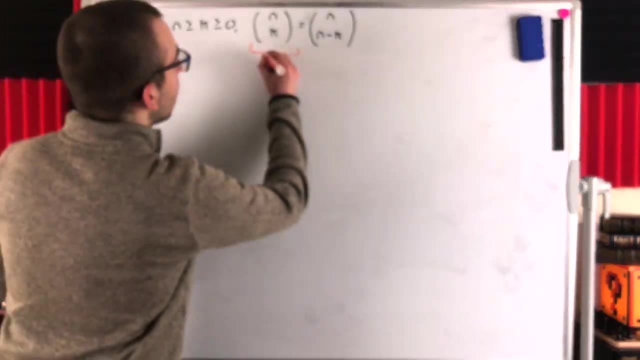 justification, which is super easy. So remember, as you just heard, this is read as: n choose k. we could call it a binomial coefficient. That's what we call them, because they give us the coefficients of binomials, which we'll see in practice in just a couple minutes. But so this? 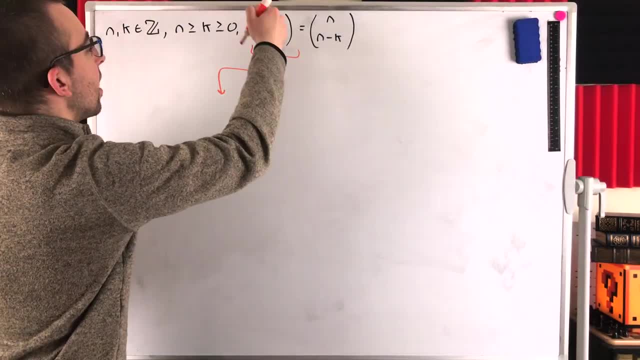 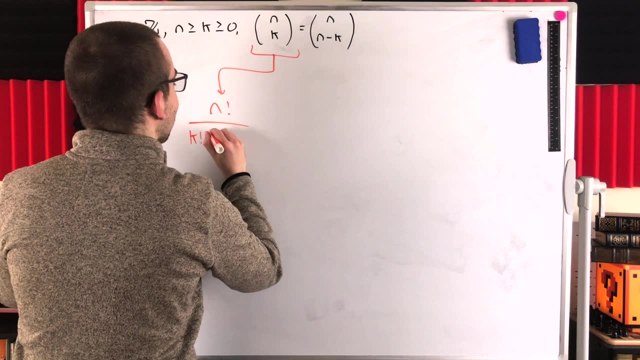 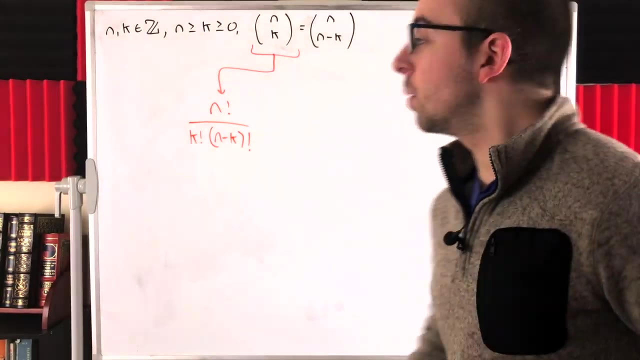 is read as n choose k, because it's the number of ways we can choose k objects from a collection of n, and it's got a nice formula. It's equal to n factorial divided by k factorial times n minus k factorial. Okay, so then what is this equal to? We want to show that the two 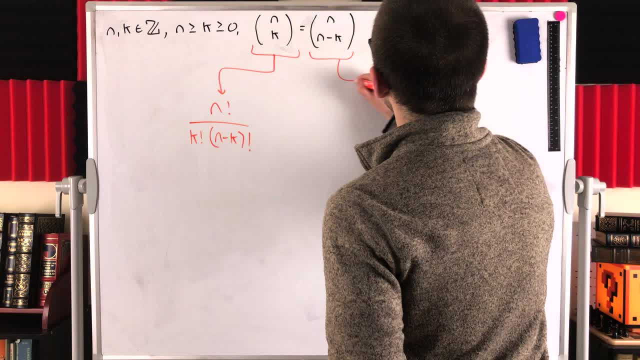 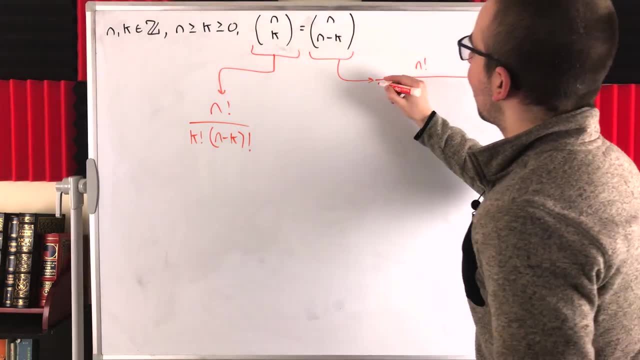 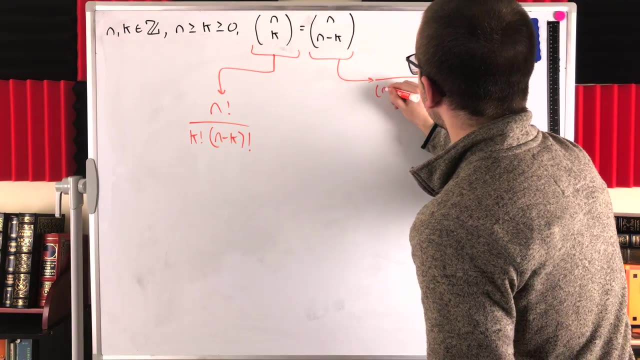 expressions are equal. Well, this thing over here, using the same formula, is equal to n factorial. might need a big fraction bar here, divided by n minus k factorial. right Over here we add k factorial. now we're going to have n minus k factorial, n minus k factorial multiplied by. 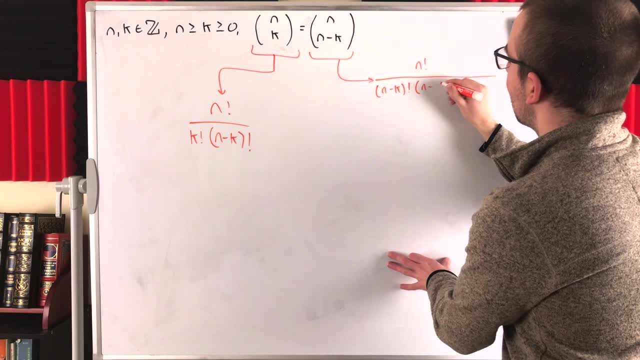 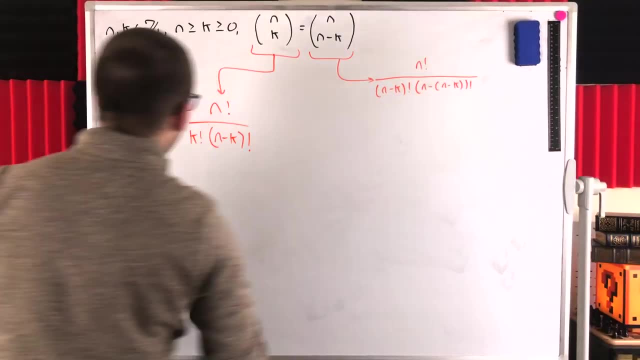 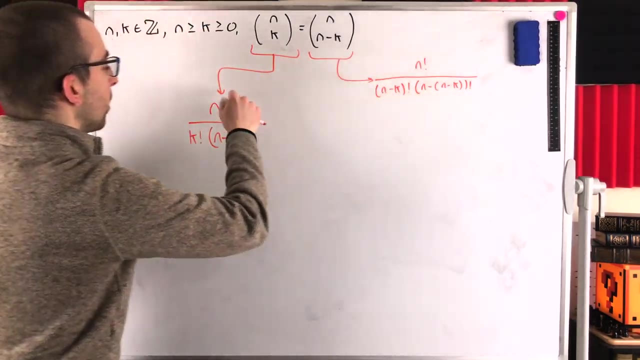 n minus n minus k. n minus n minus k- factorial. Beautiful, All right. so how do we show that this is equal to this? Well, we're already pretty close right In the numerator. we've got n- factorial, so that's good. What about the denominator? Well, we see, we've got n minus k. 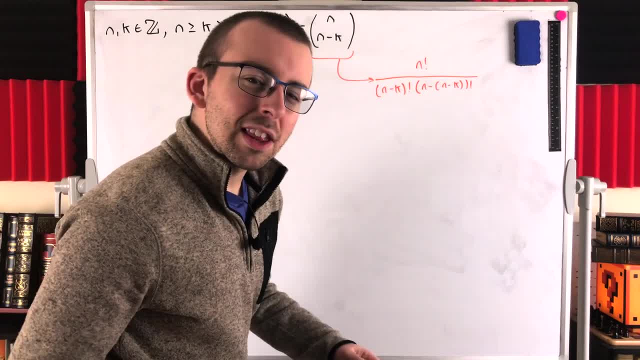 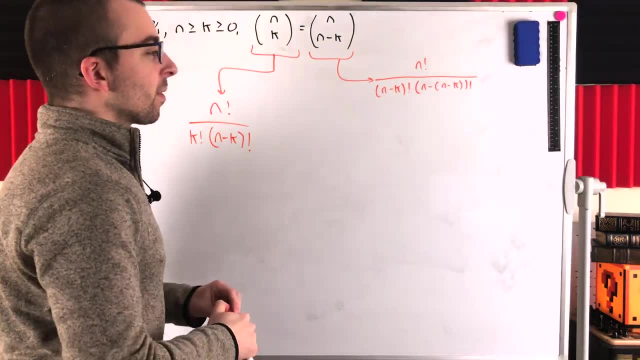 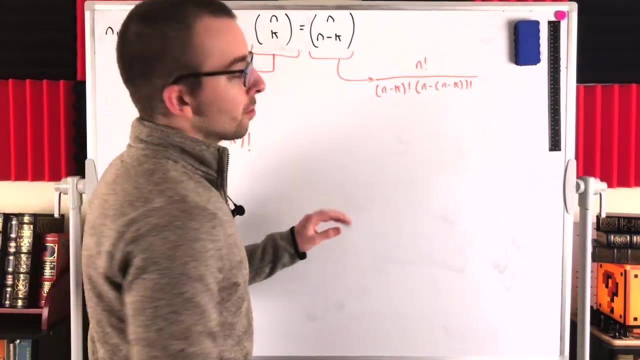 factorial, n minus k factorial. so the only things we have left to match up is the k factorial here and the n minus n minus k factorial there. Well, how can we do that? Well, it's pretty much handed to us on a silver platter. this is just k factorial, right? Check out the subtraction. 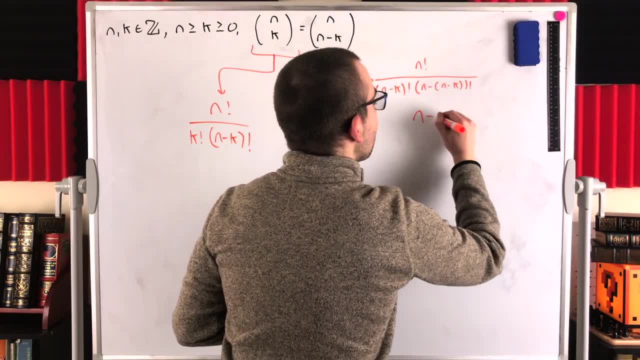 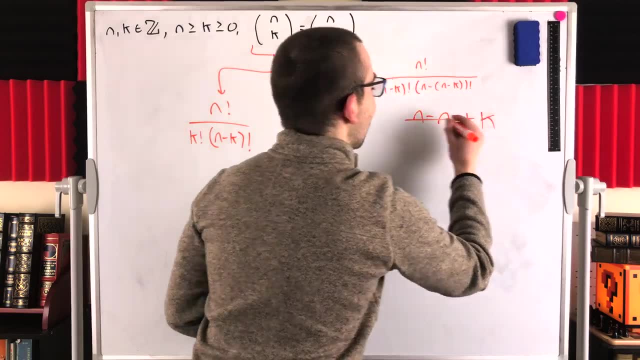 it's n minus n minus k. So when we do that out, we're going to get n minus n, which is nothing plus k, because minus minus that's a plus k, and of course this is all a factorial, And so we're just left with k factorial. look at that. that's exactly what we have over here. 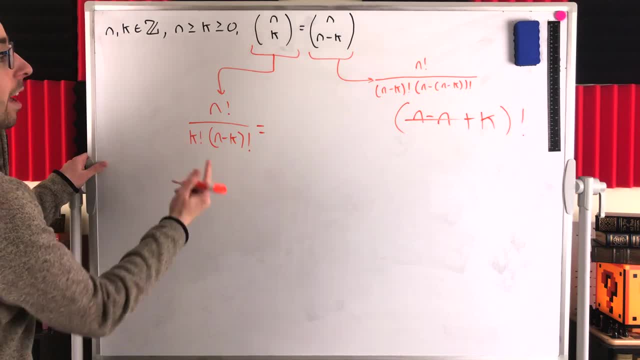 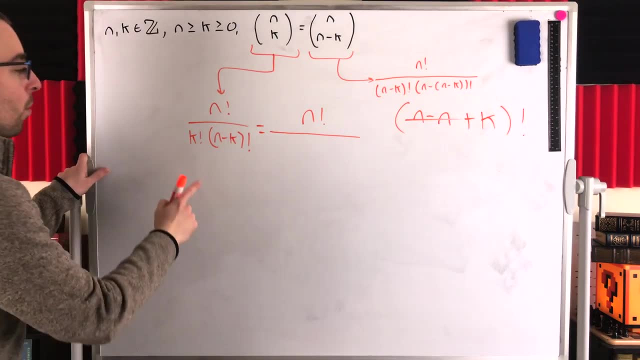 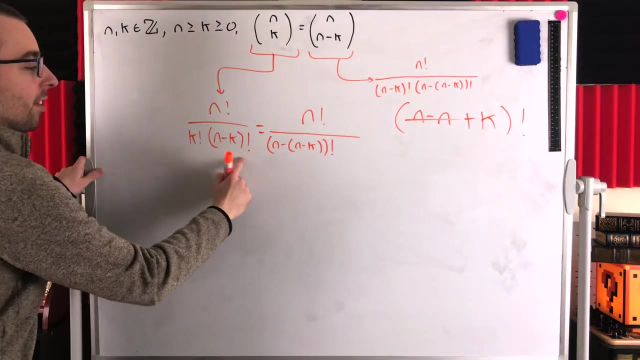 So clearly, you know, we could just rewrite k factorial as n minus n minus k factorial. so if we do that, you know, just a formality at this point- rewrite k factorial as n minus n minus k factorial, and then we've got our n minus k factorial that we had originally. 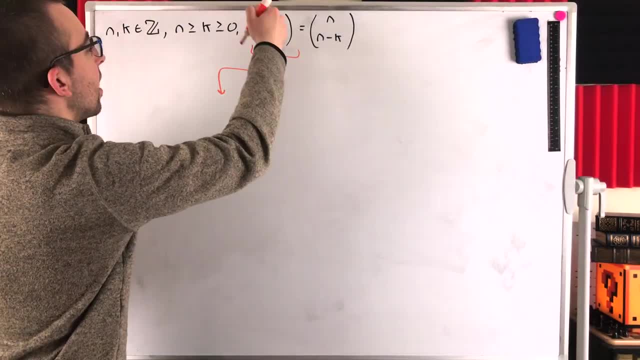 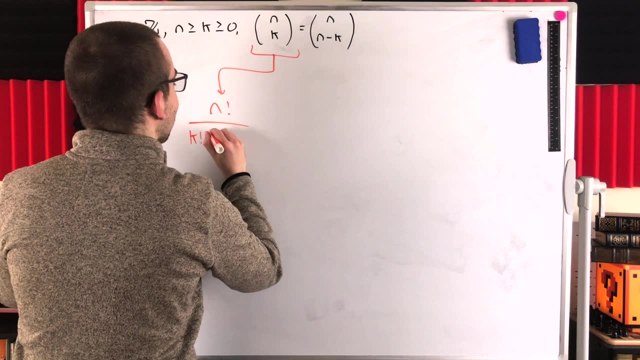 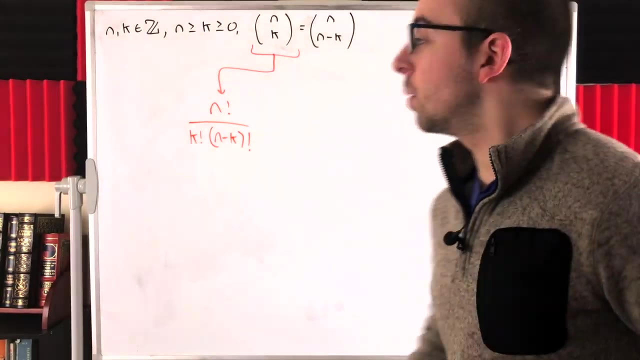 is read as n choose k, because it's the number of ways we can choose k objects from a collection of n, and it's got a nice formula. It's equal to n factorial divided by k factorial times n minus k factorial. Okay, so then what is this equal to? We want to show that the two 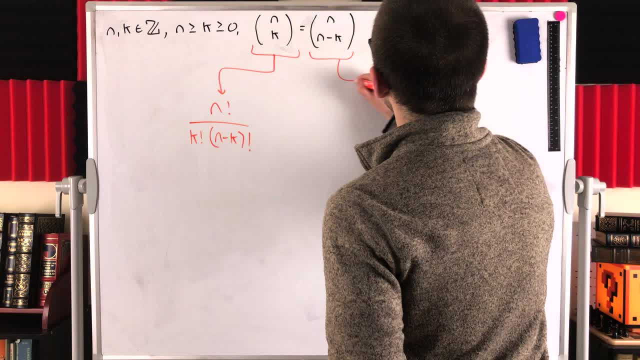 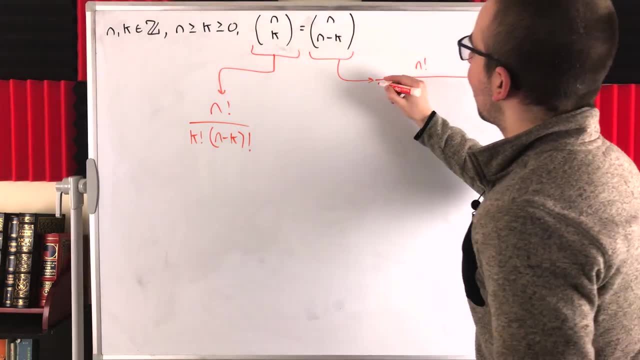 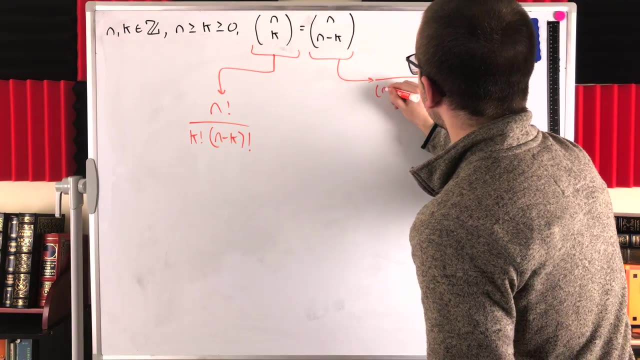 expressions are equal. Well, this thing over here, using the same formula, is equal to n factorial. might need a big fraction bar here, divided by n minus k factorial. right Over here we add k factorial. now we're going to have n minus k factorial, n minus k factorial multiplied by. 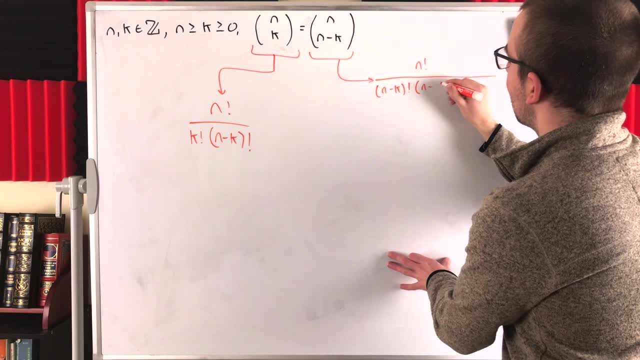 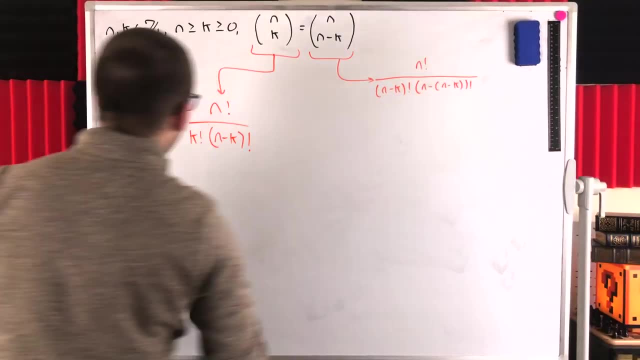 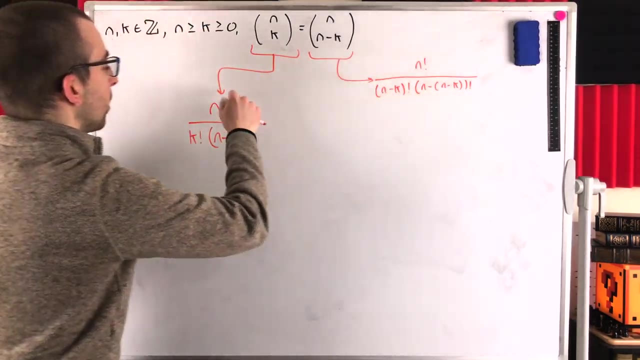 n minus n minus k. n minus n minus k- factorial. Beautiful, All right. so how do we show that this is equal to this? Well, we're already pretty close right In the numerator. we've got n- factorial, so that's good. What about the denominator? Well, we see, we've got n minus k. 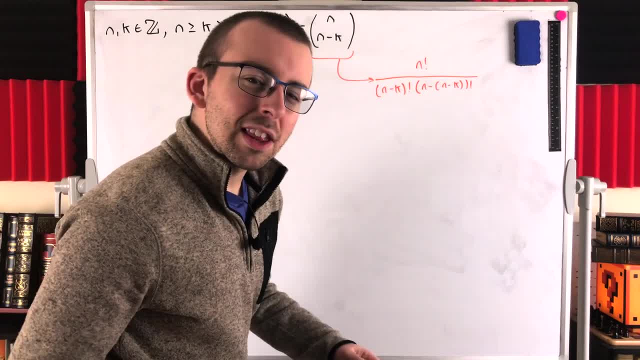 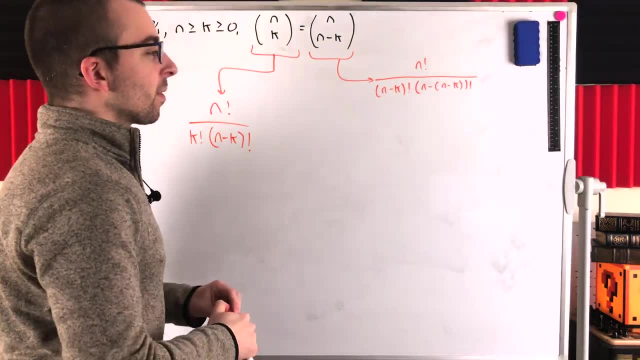 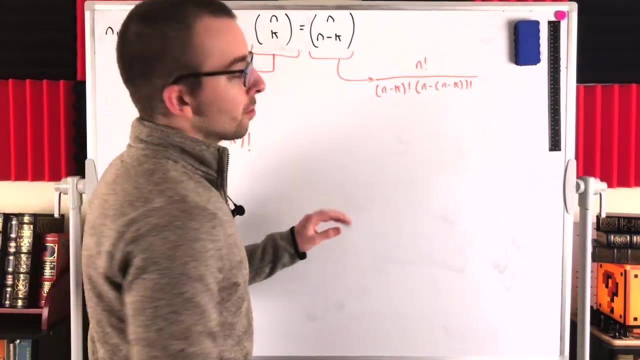 factorial, n minus k factorial. so the only things we have left to match up is the k factorial here and the n minus n minus k factorial there. Well, how can we do that? Well, it's pretty much handed to us on a silver platter. this is just k factorial, right? Check out the subtraction. 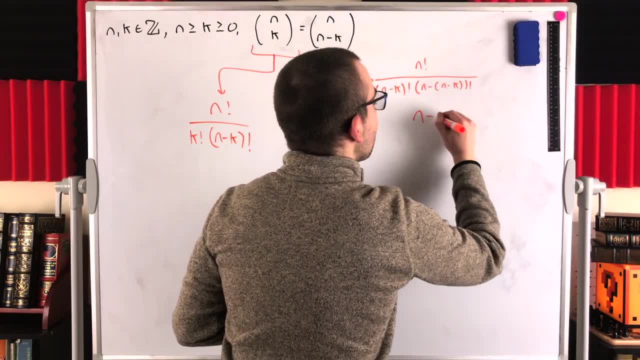 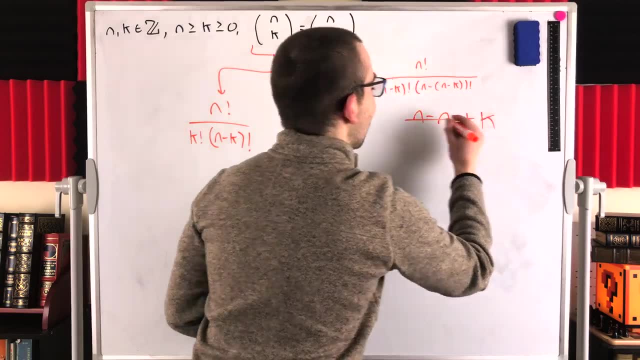 it's n minus n minus k. So when we do that out, we're going to get n minus n, which is nothing plus k, because minus minus that's a plus k, and of course this is all a factorial, And so we're just left with k factorial. look at that. that's exactly what we have over here. 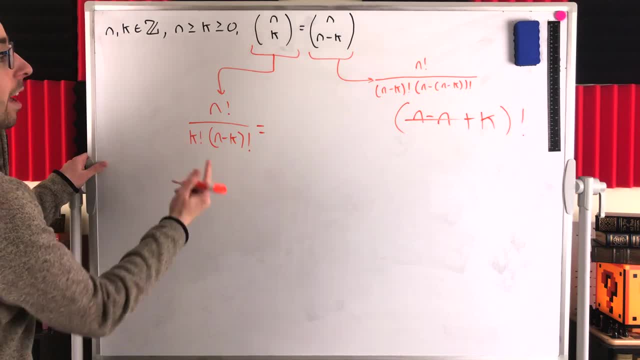 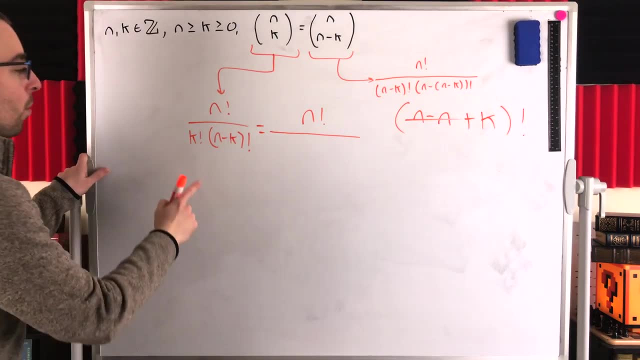 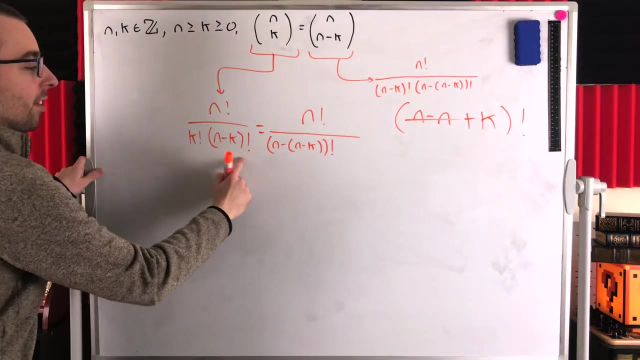 So clearly, you know, we could just rewrite k factorial as n minus n minus k factorial. so if we do that, you know, just a formality at this point- rewrite k factorial as n minus n minus k factorial, and then we've got our n minus k factorial that we had originally. 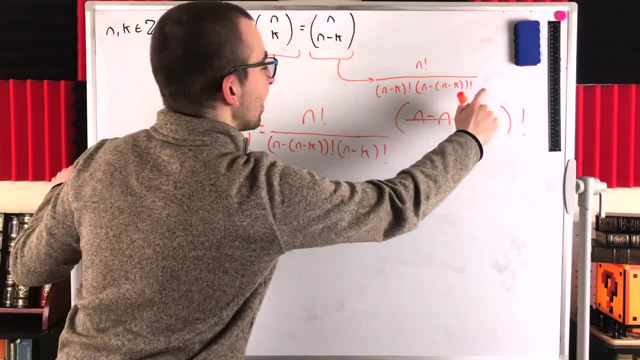 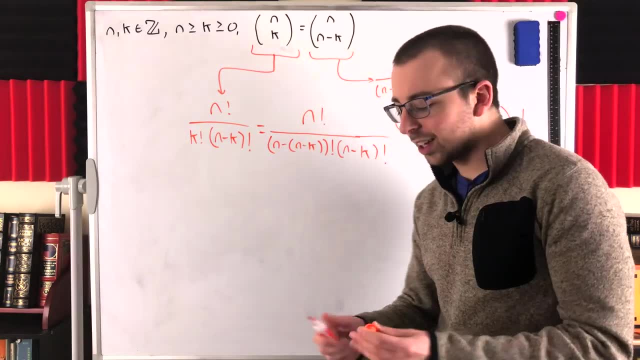 Oh, look at that. That is that We're done. That's the proof. So mathematically it's very clear. you know just One line, one line of work and you're done. So what's the intuition behind it? Why does it make? 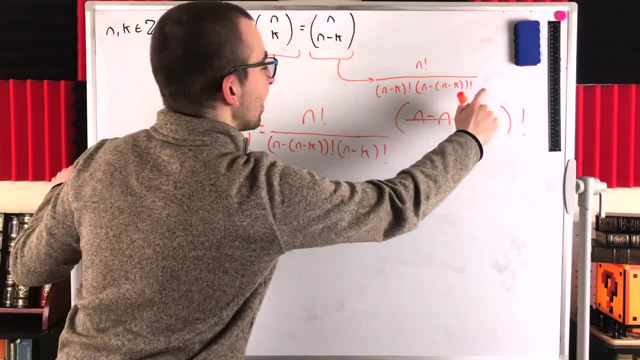 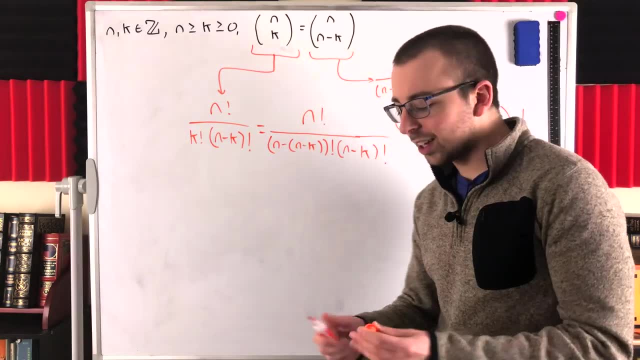 Oh, look at that. That is that We're done. That's the proof. So mathematically it's very clear. you know just One line, one line of work and you're done. So what's the intuition behind it? Why does it make? 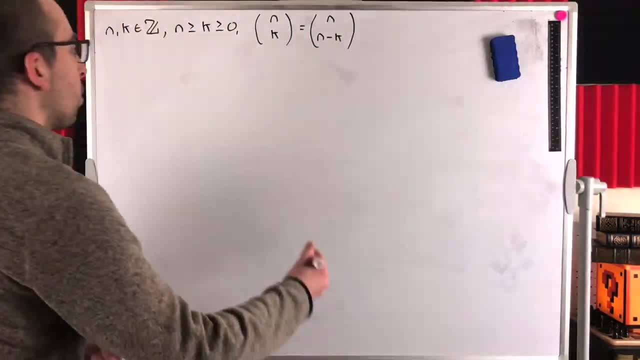 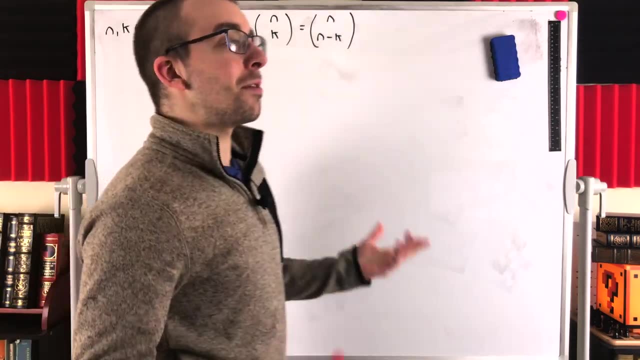 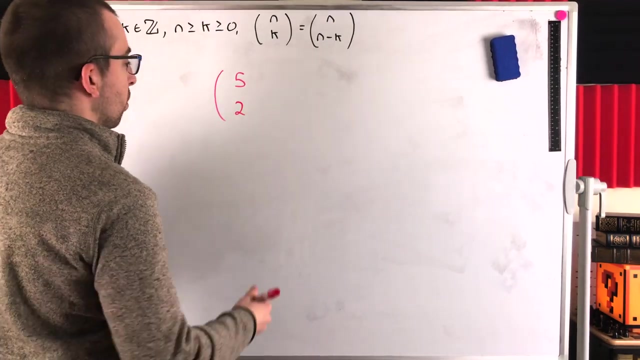 sense. Well, to see that. let's check out a super quick example. So consider, you know, maybe we've got a collection of five objects, maybe five people, So we've got a collection of five people and maybe we're selecting two to be in some sort of team, some sort of pair. five choose two And 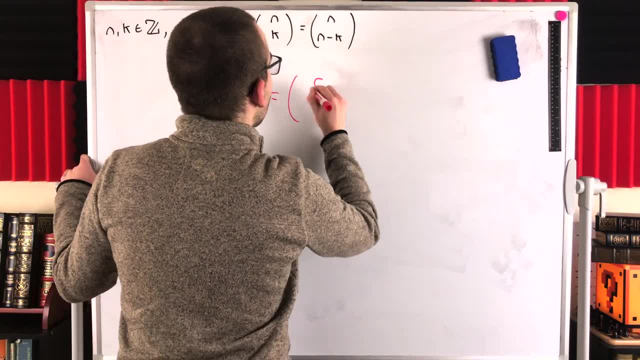 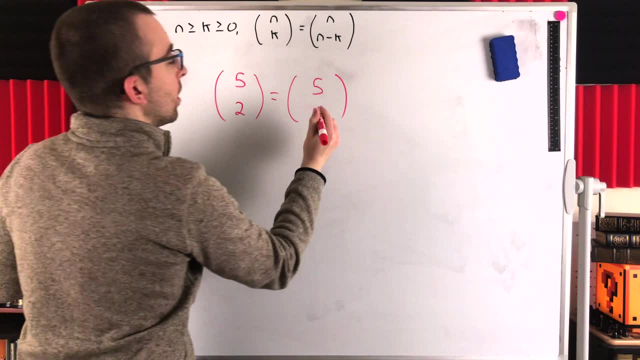 we've just shown that five choose two must be equal to five choose five minus two. I guess we'll write it out: Five choose five minus two and then let's go ahead and erase it, because we know that five minus two is three. And if we do the math, of course we'll see. 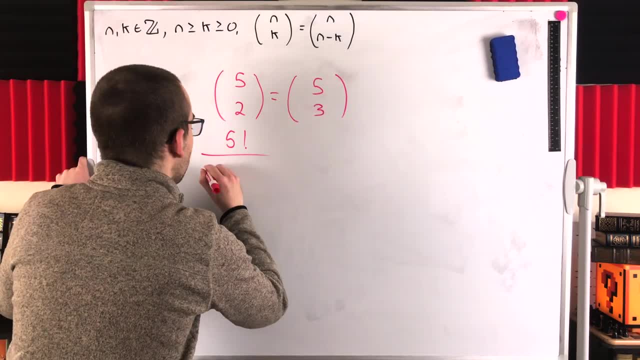 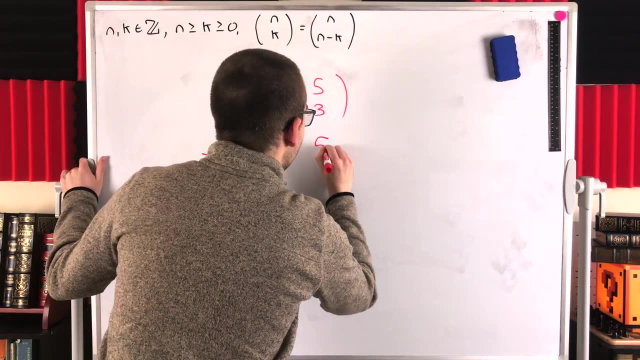 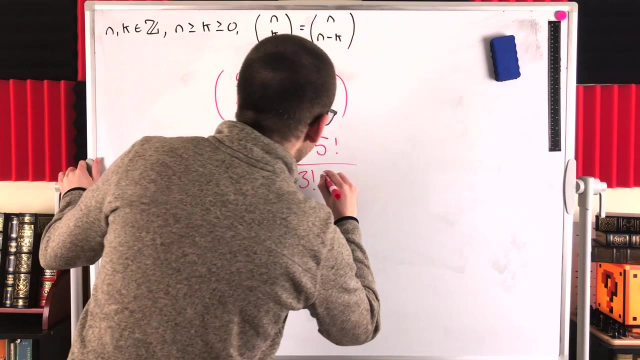 that this is certainly true. This is equal to five factorial divided by two factorial times five minus two factorial, which is three factorial. And this is equal to five factorial divided by three factorial times five minus three factorial, which is two factorial. Look at that, You know. 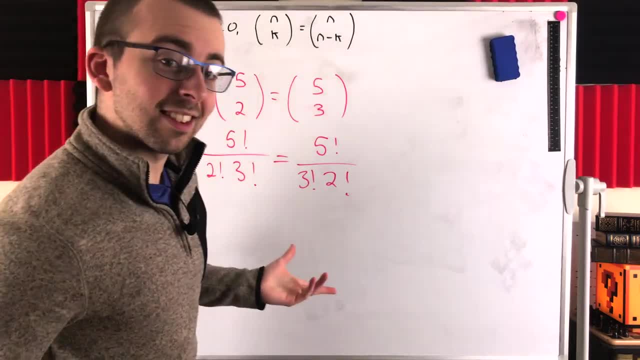 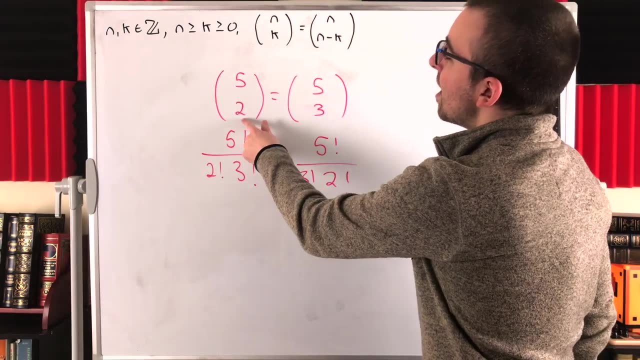 order of multiplication doesn't matter- Very clear. So why is this true? Why does it work so beautifully? Well, quite simply, because the number of ways we can pick two people- Well, here's how we got to think about it, right- The number of ways we can pick three people. 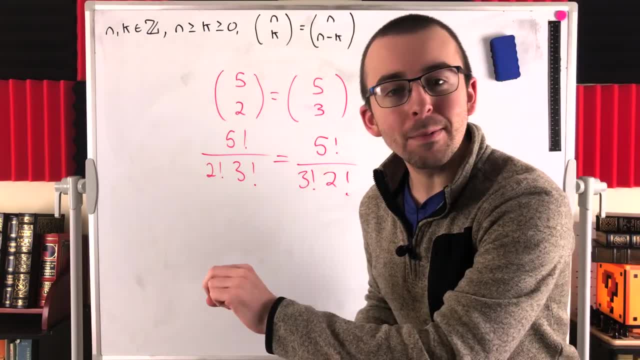 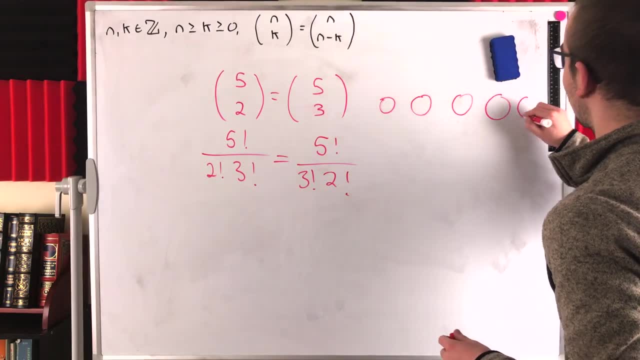 is the same as picking two people to not pick right. So imagine, you know, imagine we got our collection of. Let's see what's the worst way I can draw these stick figures: One, two, three, four, five, boom. 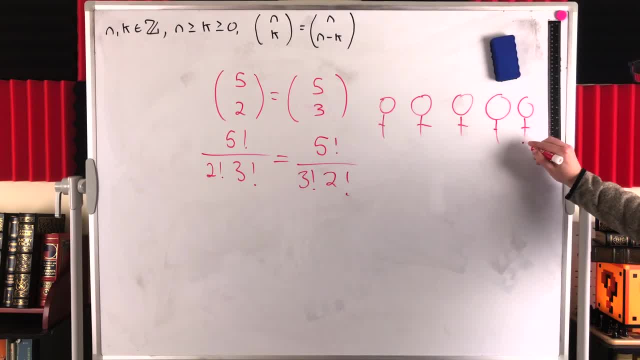 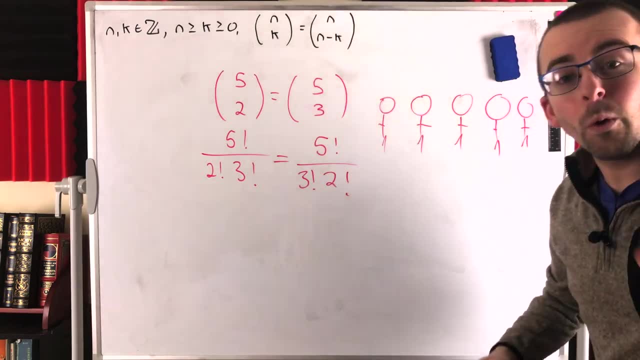 Boom, boom, boom, boom, Bop, bop, bop, bop, bop, And we got some Vs for the legs, Beautiful. So you know we could pick three. right, Let's pick these guys, these three here, Or equivalently. 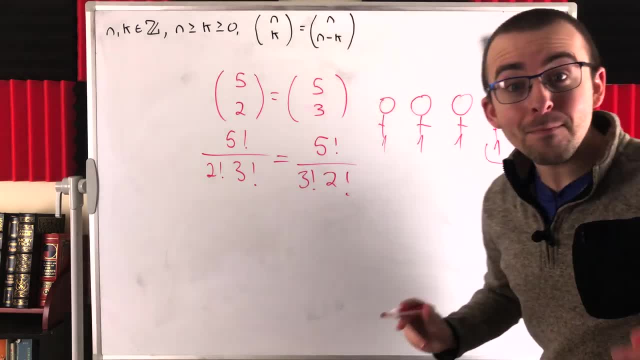 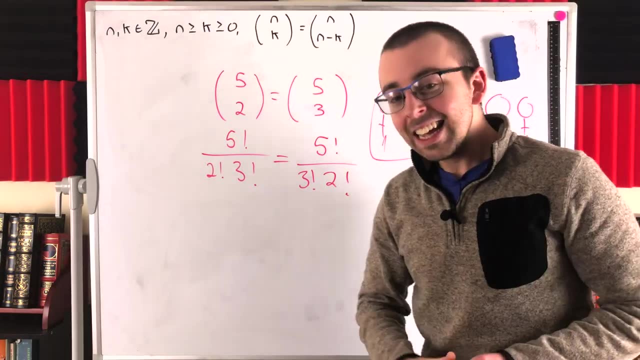 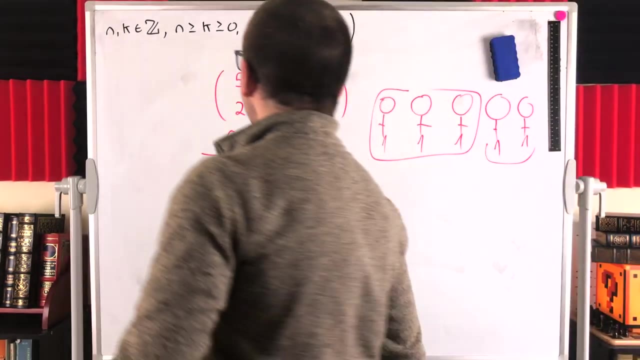 we could choose two people to not pick, And if we choose these two people to not pick, that means we're going to pick these three people. So every time we choose two people, that's the same as not picking the other three people. So, of course, 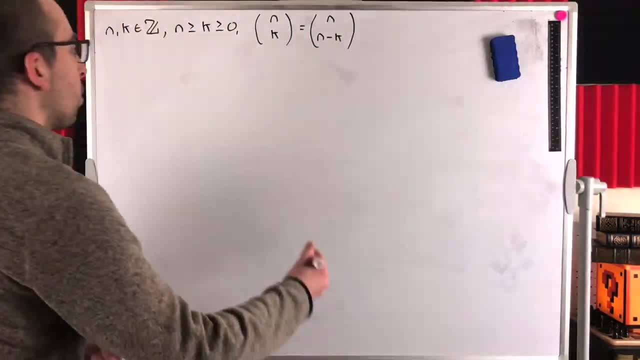 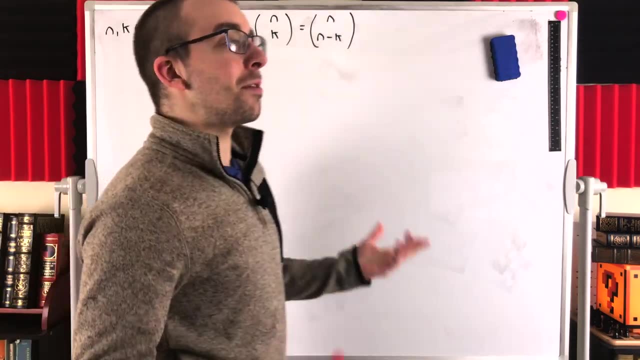 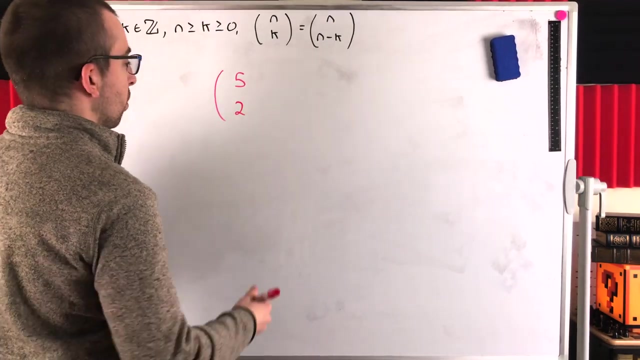 sense. Well, to see that. let's check out a super quick example. So consider, you know, maybe we've got a collection of five objects, maybe five people, So we've got a collection of five people and maybe we're selecting two to be in some sort of team, some sort of pair. five choose two And 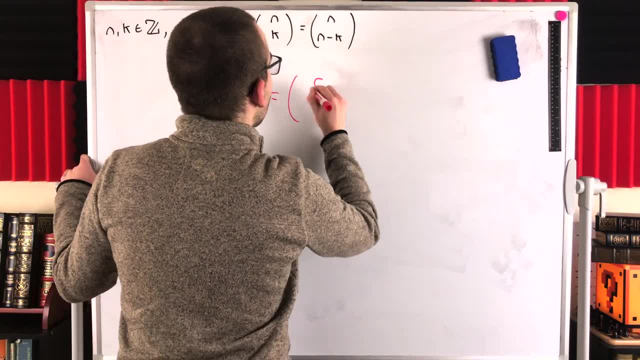 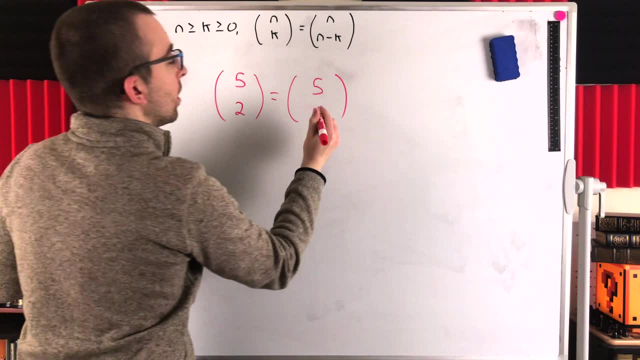 we've just shown that five choose two must be equal to five choose five minus two. I guess we'll write it out: Five choose five minus two and then let's go ahead and erase it, because we know that five minus two is three. And if we do the math, of course we'll see. 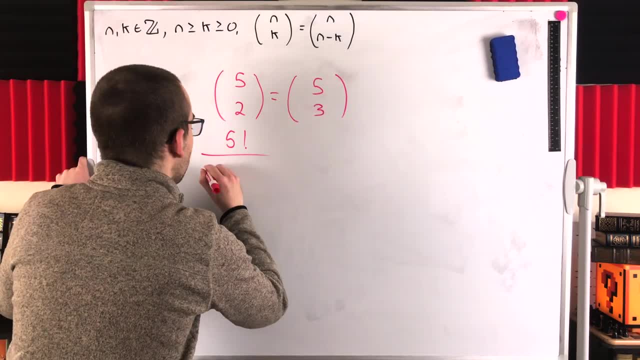 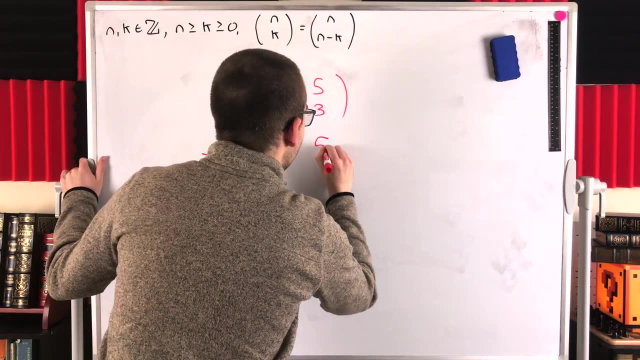 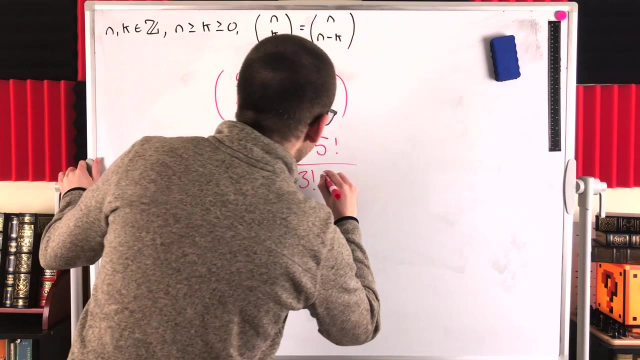 that this is certainly true. This is equal to five factorial divided by two factorial times five minus two factorial, which is three factorial. And this is equal to five factorial divided by three factorial times five minus three factorial, which is two factorial. Look at that, You know. 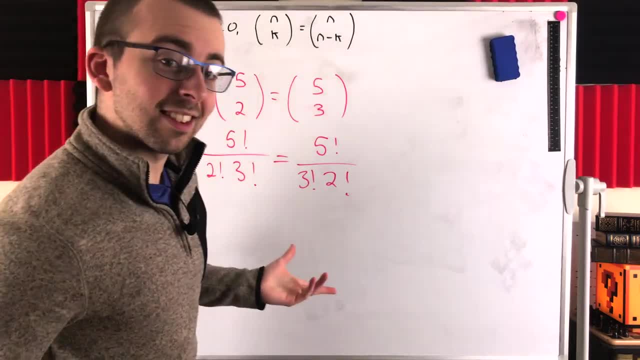 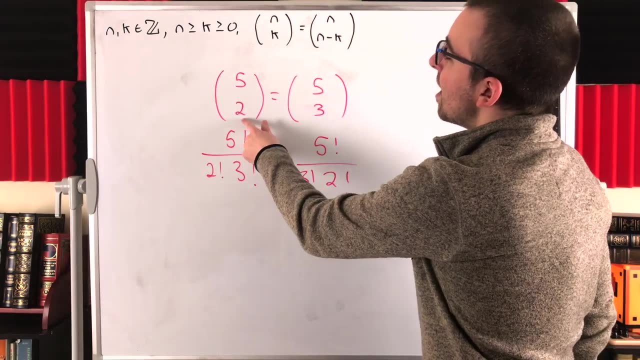 order of multiplication doesn't matter- Very clear. So why is this true? Why does it work so beautifully? Well, quite simply, because the number of ways we can pick two people- Well, here's how we got to think about it, right- The number of ways we can pick three people. 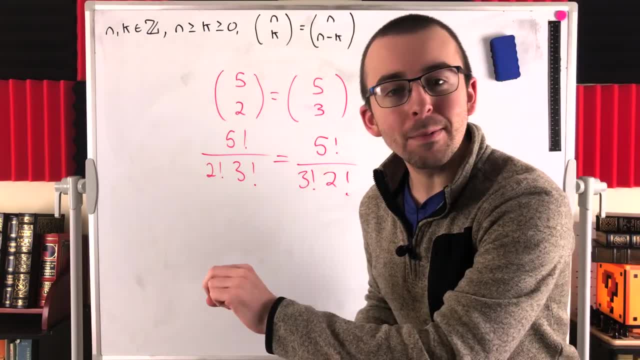 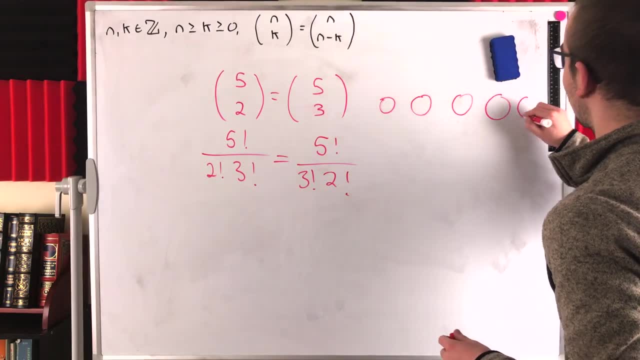 is the same as picking two people to not pick right. So imagine, you know, imagine we got our collection of. Let's see what's the worst way I can draw these stick figures: One, two, three, four, five, boom. 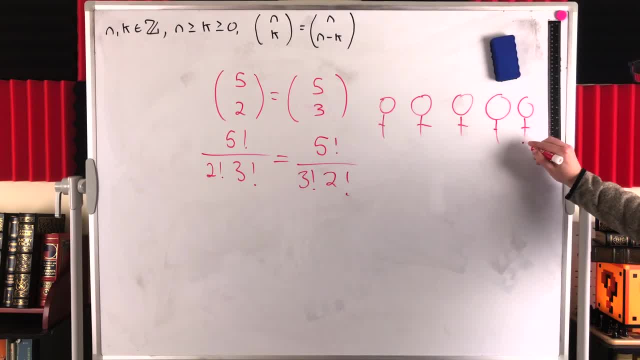 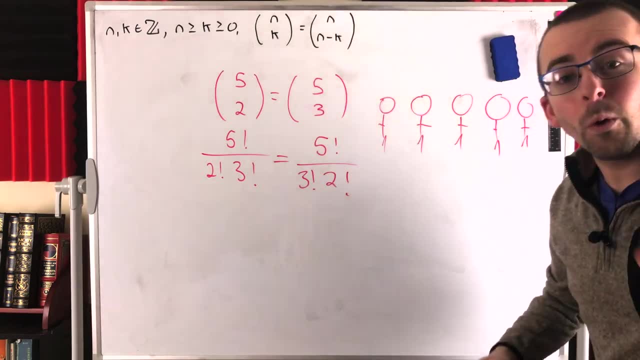 Boom, boom, boom, boom, Bop, bop, bop, bop, bop, And we got some Vs for the legs, Beautiful. So you know we could pick three. right, Let's pick these guys, these three here, Or equivalently. 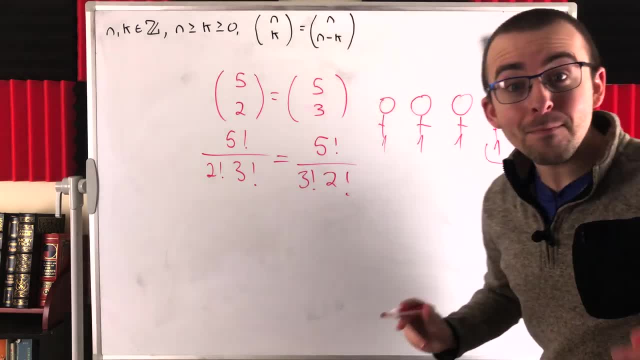 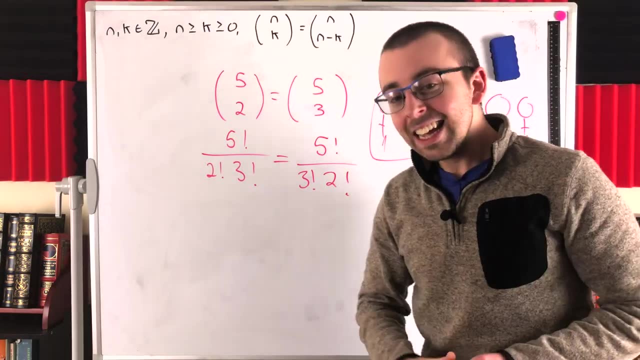 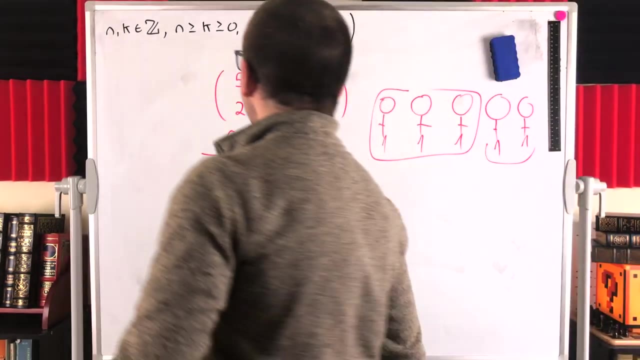 we could choose two people to not pick, And if we choose these two people to not pick, that means we're going to pick these three people. So every time we choose two people, that's the same as not picking the other three people. So, of course, 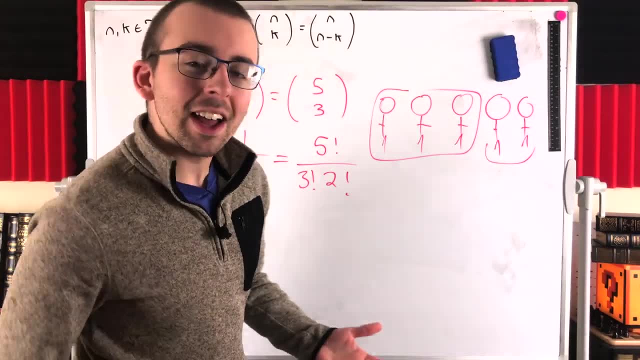 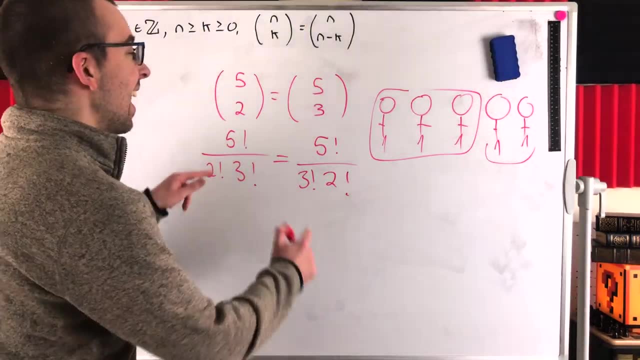 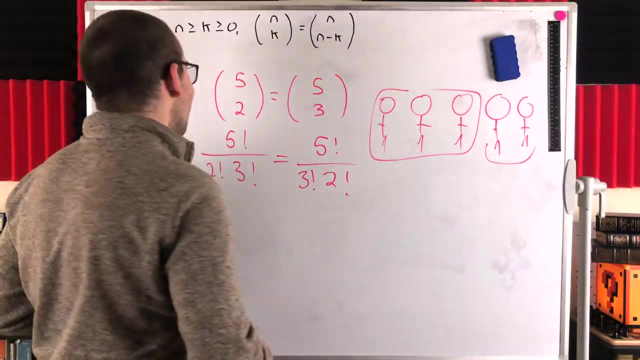 the number of ways we can choose two people from a collection of five is the same as the number of ways that we can choose three people from a collection of five, Because, again, every time we pick two people, we've implicitly chosen three people to not pick. Hopefully that makes sense. 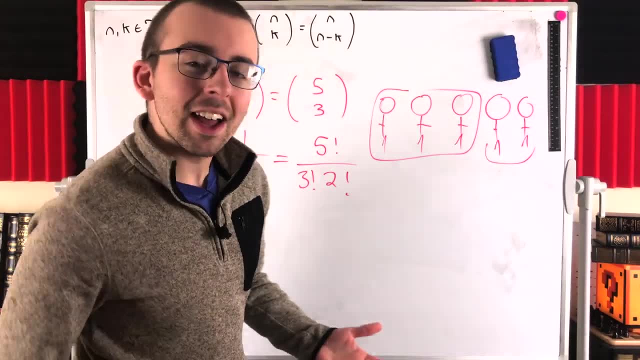 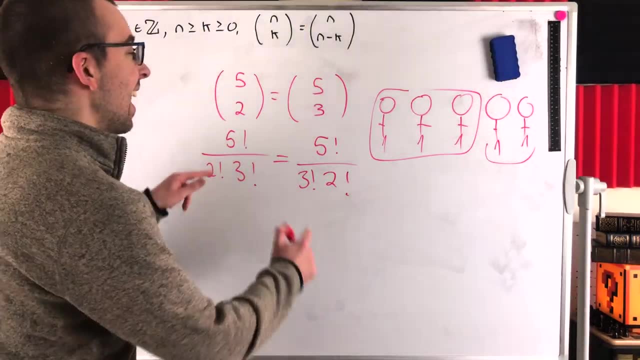 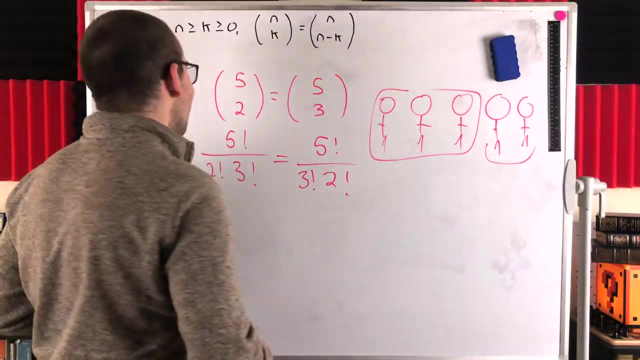 the number of ways we can choose two people from a collection of five is the same as the number of ways that we can choose three people from a collection of five, Because, again, every time we pick two people, we've implicitly chosen three people to not pick. Hopefully that makes sense. 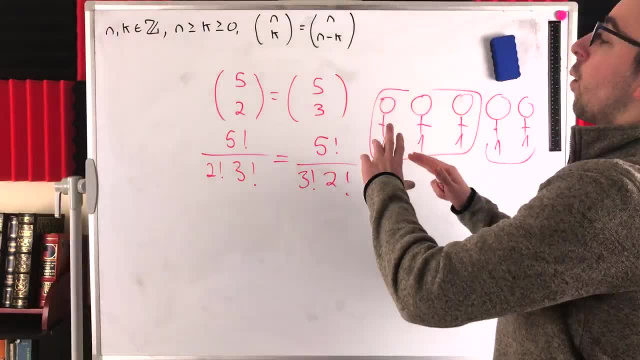 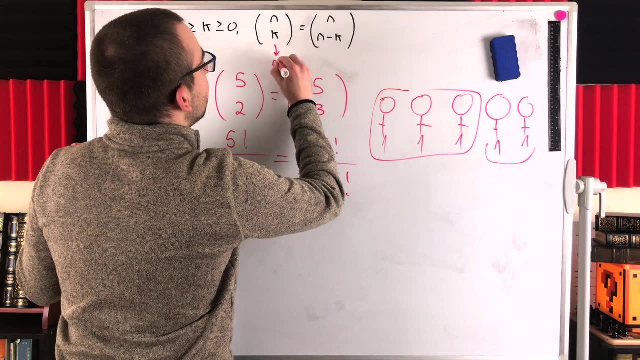 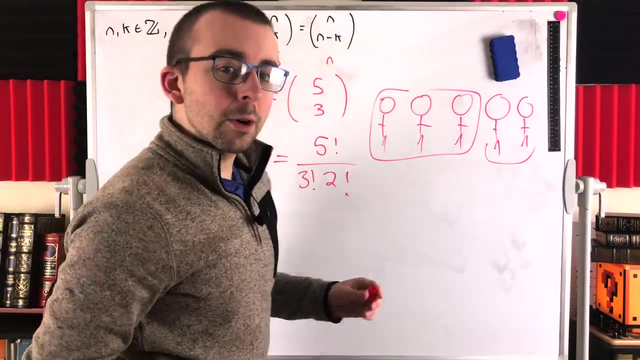 I think it's pretty neat, It's pretty beautiful, And of course we call this symmetric, a symmetric property, because the lowest value we can have down here is zero, right, And the highest value is n, So this bottom value can range from zero to n, And so we're saying this is symmetric. 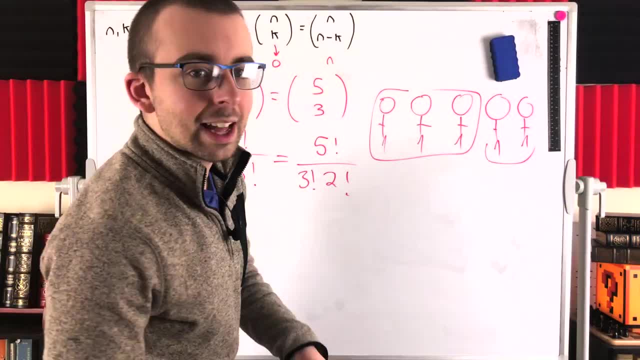 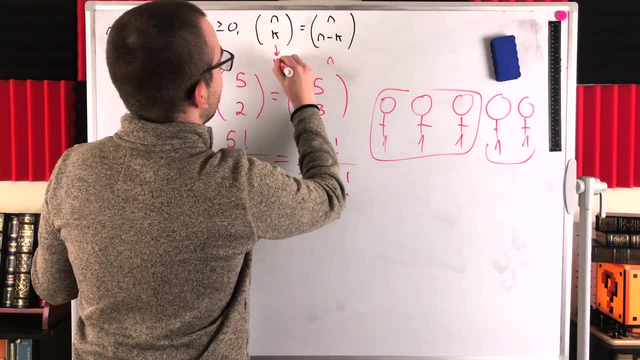 because if we go up k from the lowest possible value zero, that's the same as going down k from the highest possible value n. In other words, if we have k in there, that's the same as having n minus k in there. So hopefully you can sort of see those shapes you know. 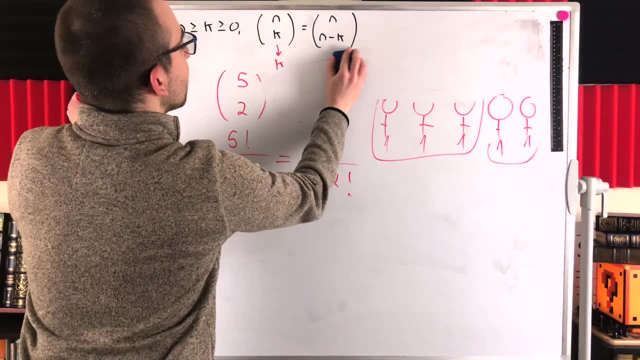 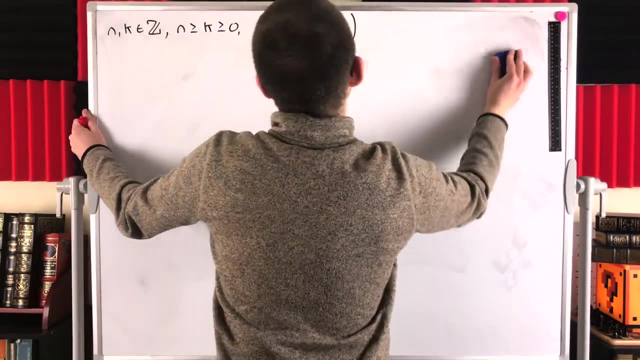 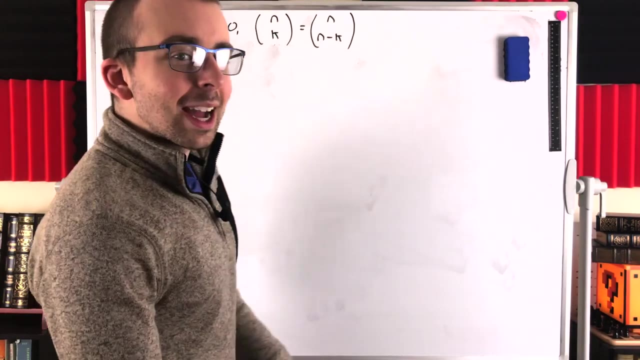 why we would call that symmetric. But even more clearly we can see it if we check out the expansion of a binomial, which is one of the places this really comes in handy. You got your binomial theorem. you got your symmetric property of the binomial coefficient. 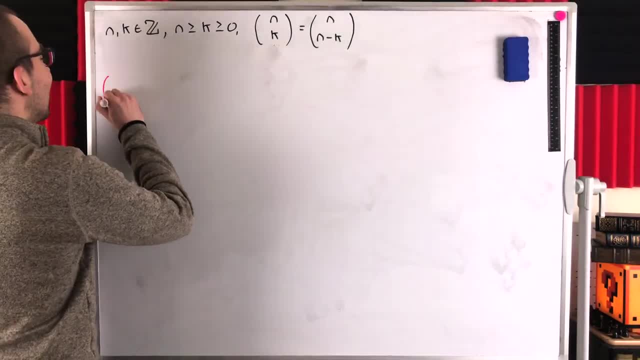 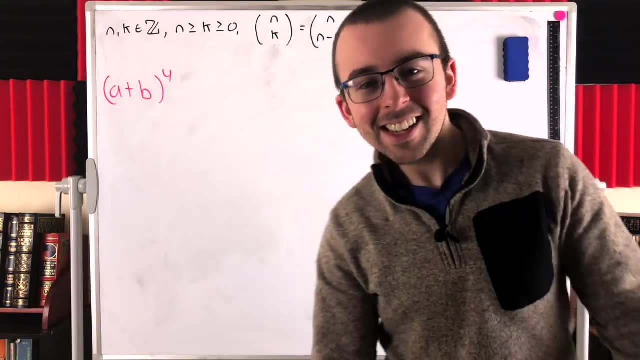 bam, bam bam. you're good to go. Say we have. so say we've got this binomial right- A plus b- to the power of four. If we had a plus b squared, we can do that right Easy peasy. A plus b cubed. 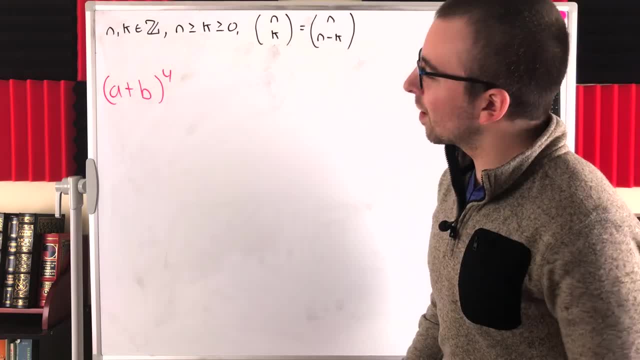 easy enough. Maybe we'll just do it by hand. But a plus b to the fourth, a plus b to the fifth, sixth, seventh, you start getting up there. You're like: yeah, give me the binomial theorem I've had. 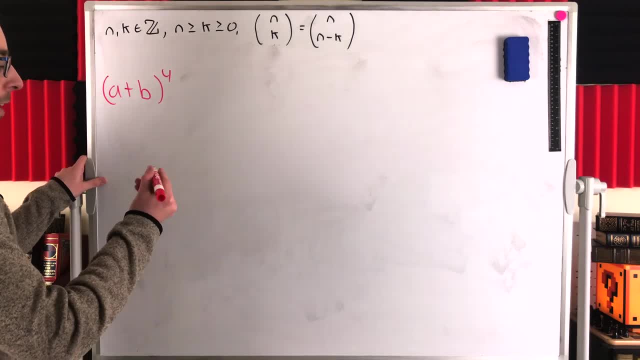 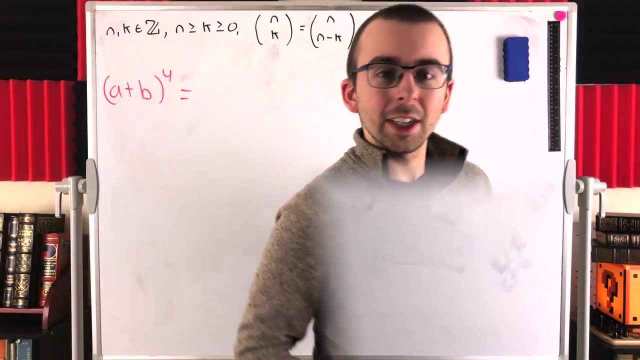 enough of this business without the binomial theorem, you know. So we apply the binomial theorem, And the binomial theorem tells us that we can expand this very easily, very beautifully. And here's how we do it right: We start with our exponent four, choose zero, And then we're. 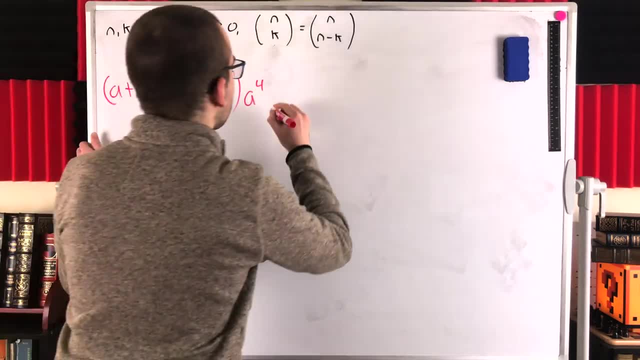 going to have our first term: a to the power of four, b to the power of zero, so we don't have to write it. And then we just increment everything up, up and down, right? So four, choose one now. 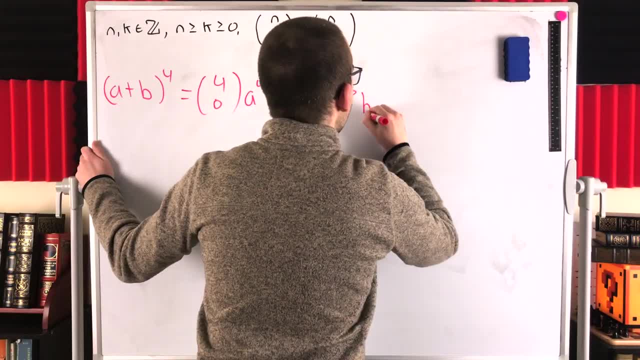 plus a to the power of zero. And then we just increment everything up, up and down, right. So a a is going to go down, so a to the power of three multiplied by b. Now b's gone up from b to. 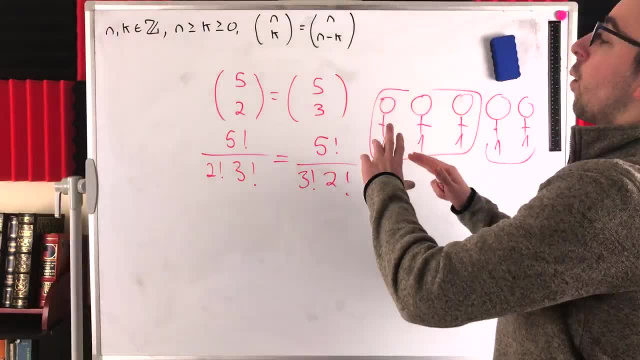 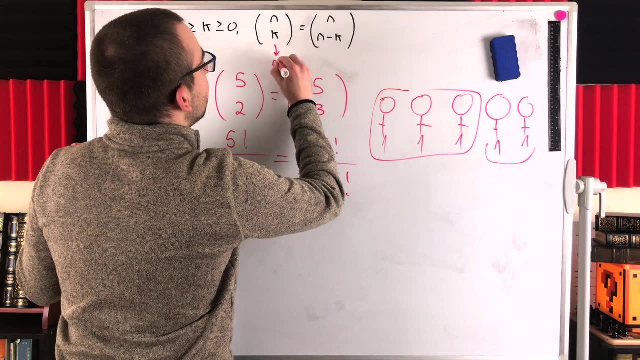 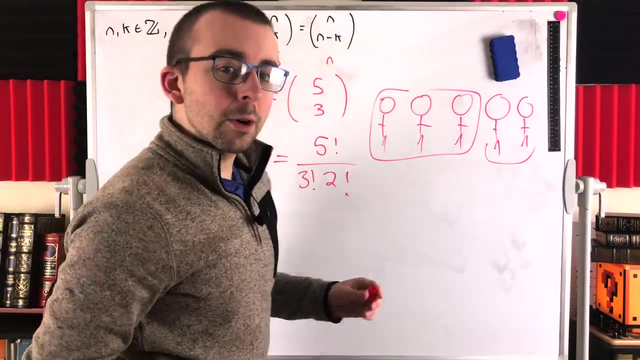 I think it's pretty neat, It's pretty beautiful, And of course we call this symmetric, a symmetric property, because the lowest value we can have down here is zero, right, And the highest value is n, So this bottom value can range from zero to n, And so we're saying this is symmetric. 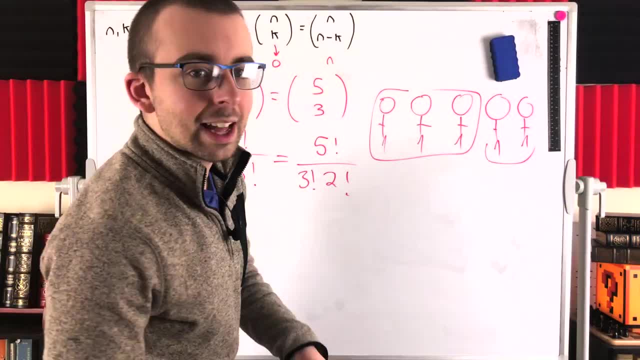 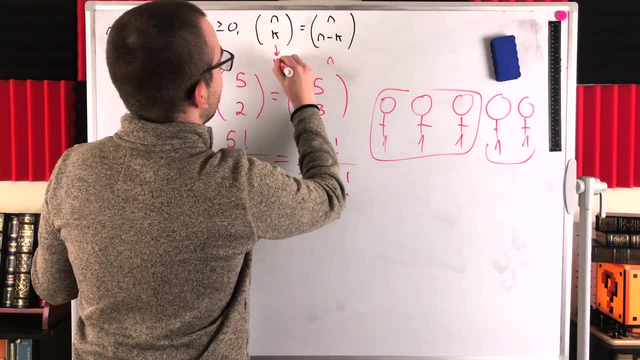 because if we go up k from the lowest possible value zero, that's the same as going down k from the highest possible value n. In other words, if we have k in there, that's the same as having n minus k in there. So hopefully you can sort of see those shapes you know. 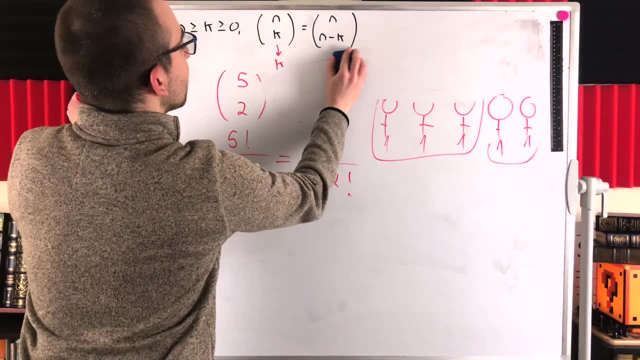 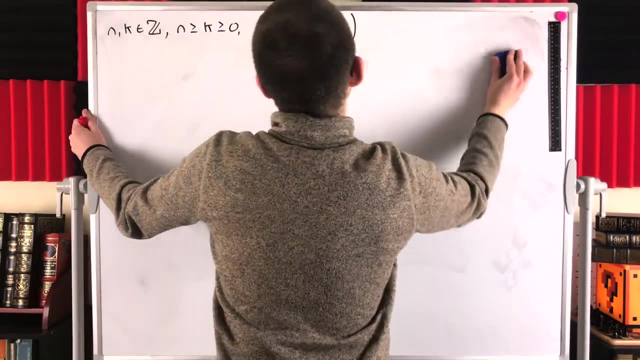 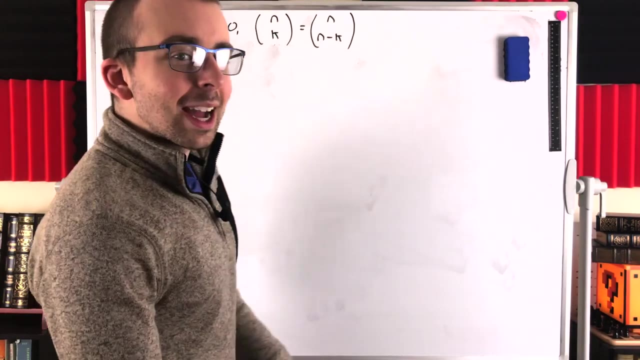 why we would call that symmetric. But even more clearly we can see it if we check out the expansion of a binomial, which is one of the places this really comes in handy. You got your binomial theorem. you got your symmetric property of the binomial coefficient. 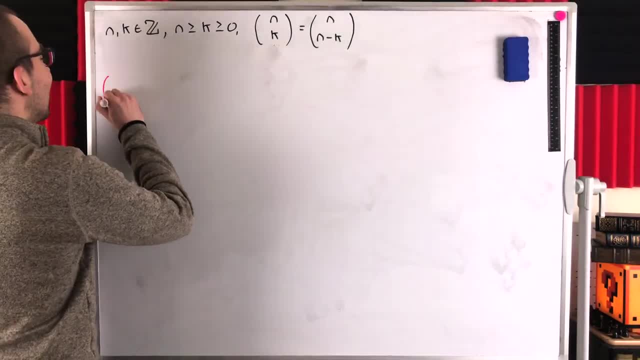 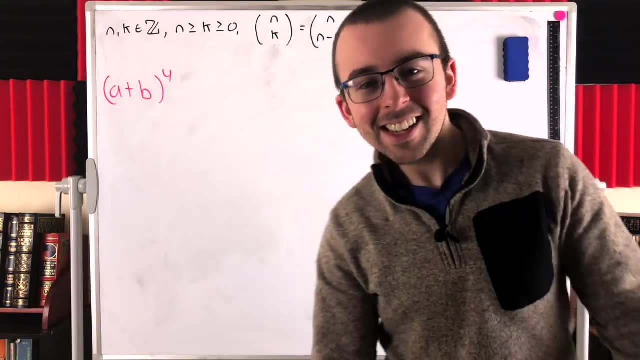 bam, bam bam. you're good to go. Say we have. so say we've got this binomial right- A plus b- to the power of four. If we had a plus b squared, we can do that right Easy peasy. A plus b cubed. 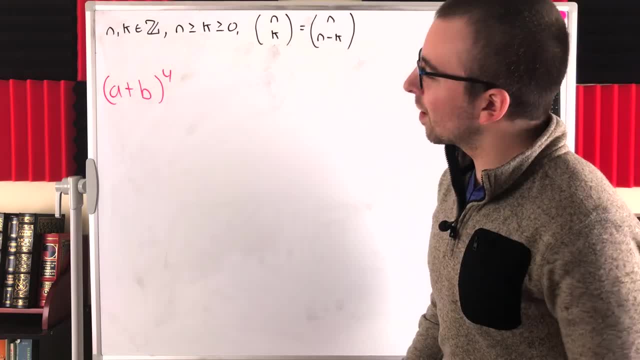 easy enough. Maybe we'll just do it by hand. But a plus b to the fourth, a plus b to the fifth, sixth, seventh, you start getting up there. You're like: yeah, give me the binomial theorem I've had. 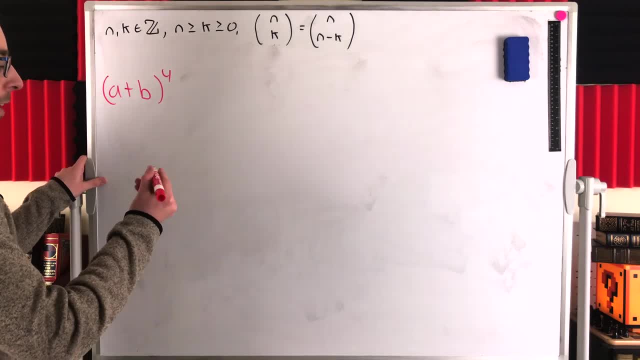 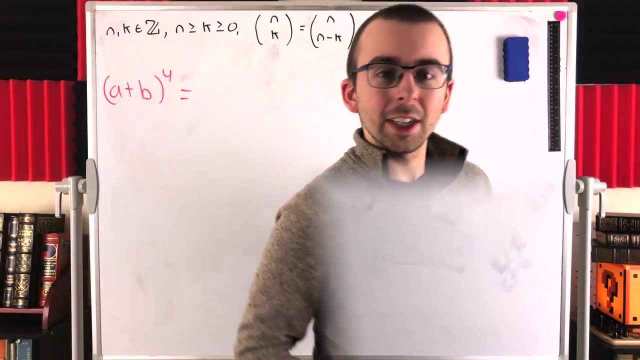 enough of this business without the binomial theorem, you know. So we apply the binomial theorem, And the binomial theorem tells us that we can expand this very easily, very beautifully. And here's how we do it right: We start with our exponent four, choose zero, And then we're. 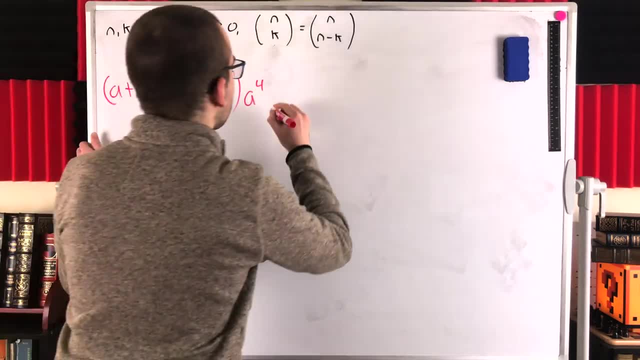 going to have our first term: a to the power of four, b to the power of zero, so we don't have to write it. And then we just increment everything up, up and down, right? So four, choose one now. 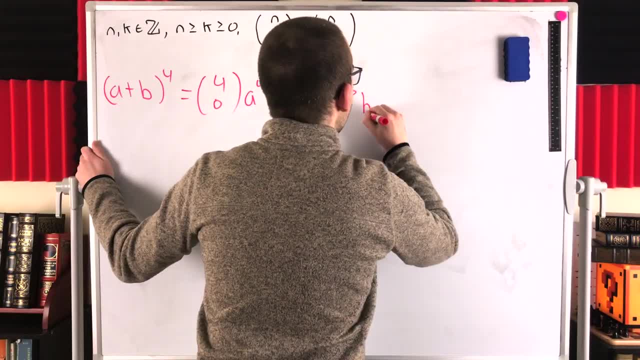 plus a to the power of zero. And then we just increment everything up, up and down, right. So a a is going to go down, so a to the power of three multiplied by b. Now b's gone up from b to. 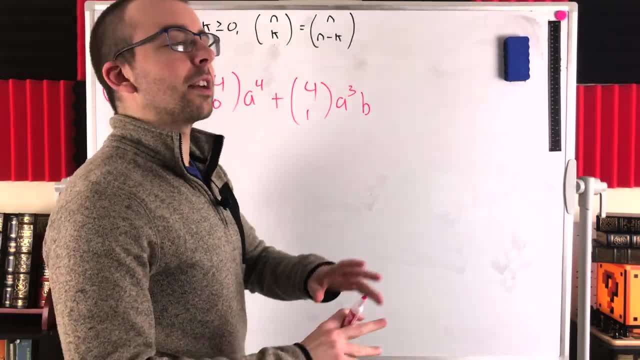 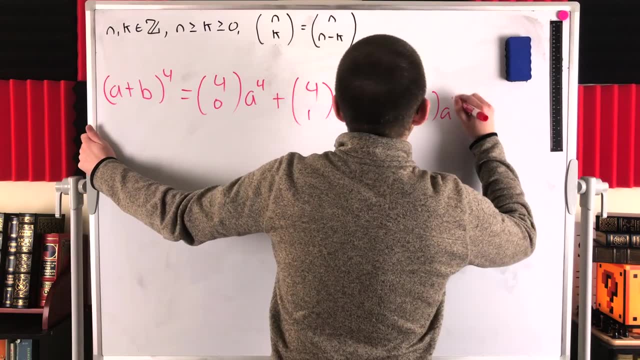 the power of zero to b to the power of one. I'm going through this super quickly because the binomial theorem is not the focus of this video. Okay, we continue incrementing. So four choose two. a goes down to a squared, b goes up to b squared. Then we've got four choose three. 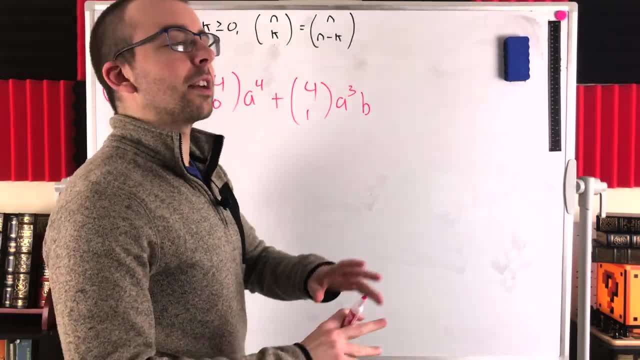 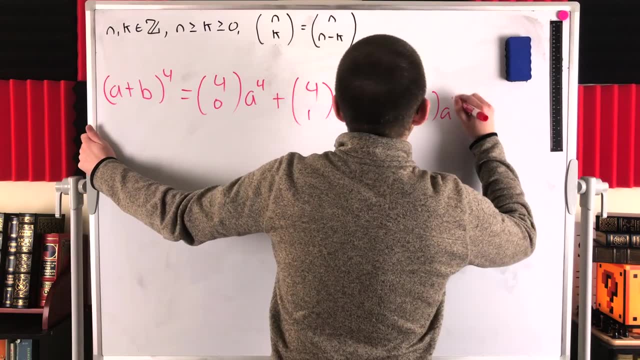 the power of zero to b to the power of one. I'm going through this super quickly because the binomial theorem is not the focus of this video. Okay, we continue incrementing. So four choose two. a goes down to a squared, b goes up to b squared. Then we've got four choose three. 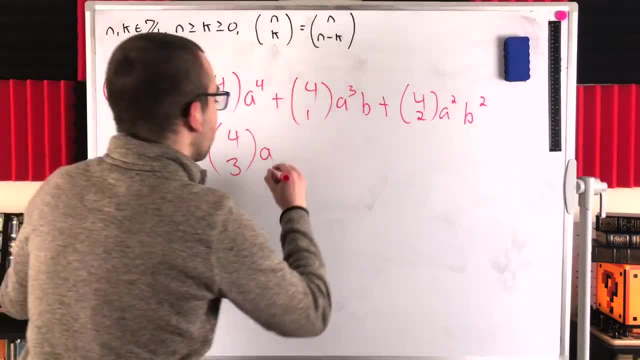 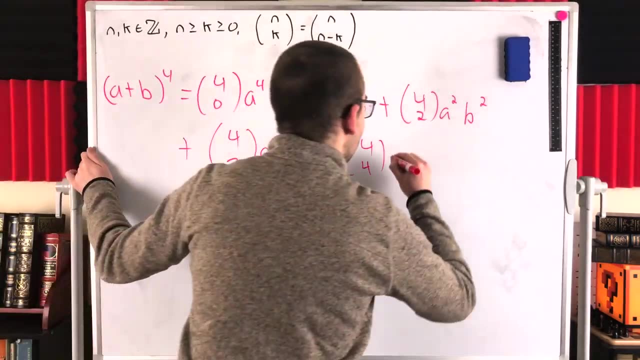 four, choose three. and then a goes down to a to the power of one, b goes up to b. cubed plus four, choose four. a goes down to a to the power of zero- that's one, we don't write it. b goes up to b to the power of four. Beautiful I could have made. 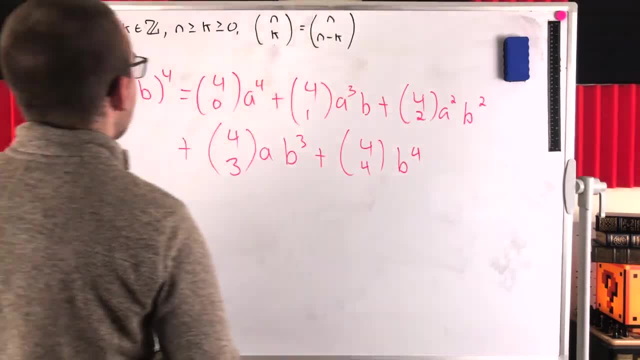 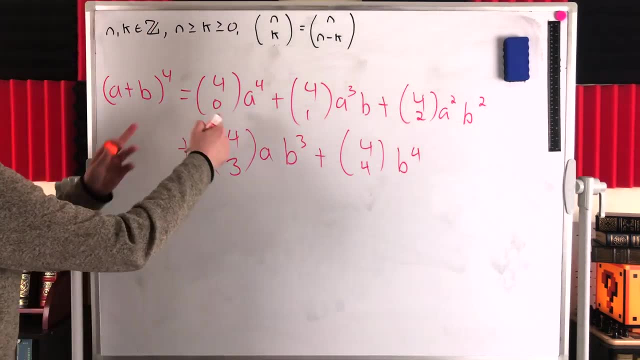 this more revealing if I had drawn everything smaller. but what are you going to do? Okay? so then say, we want to calculate the binomial coefficients here, and I've worked with these a lot. Good chance you have too. You might know some of these by heart, right? So four choose. 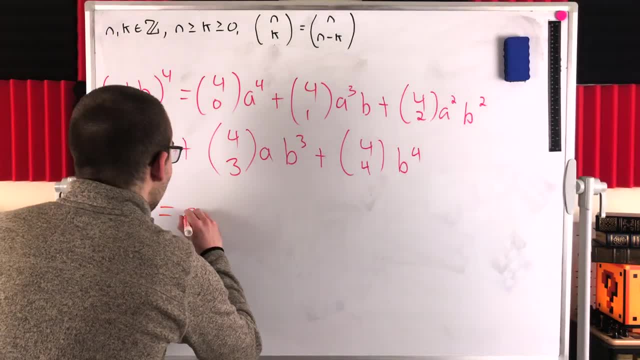 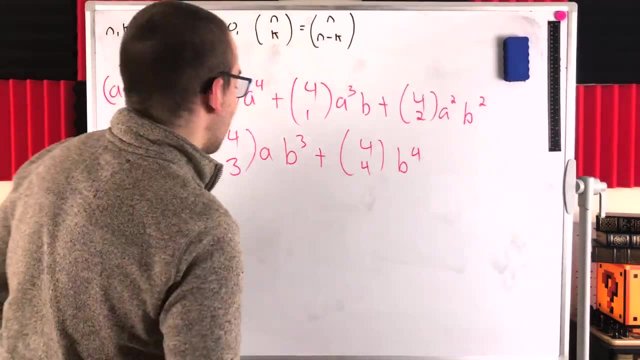 zero. What's that? Well, that's one. There's only one way. we can choose nothing. So we've got a to the power of four. Number of ways we can choose One object from four objects, that's four. So this is four, a cubed, And of course you could. 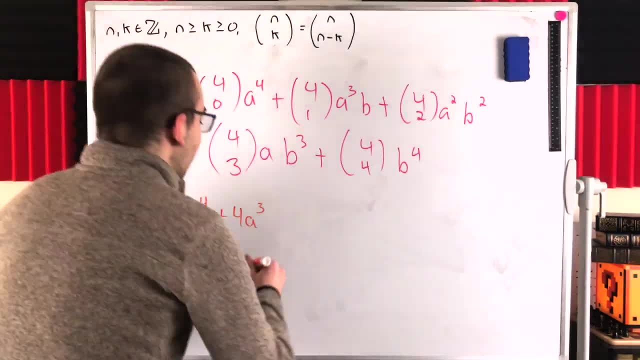 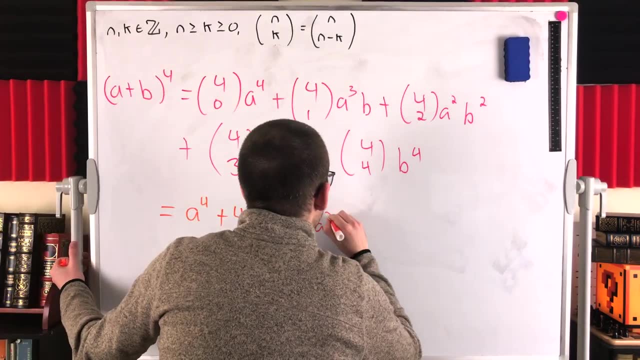 you know, use the formula here if you weren't familiar with these values. So it's four: a cubed times b, And then we've got four. choose two. that's a classic. that's six: a squared, b squared. 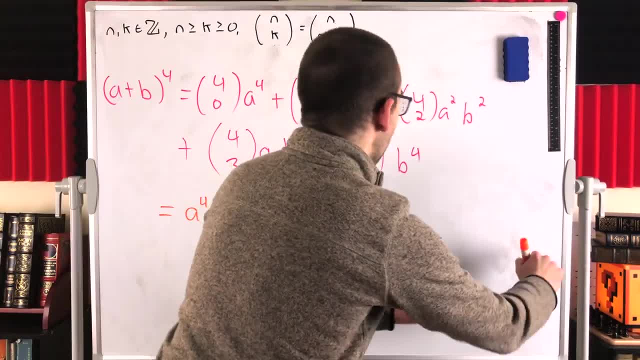 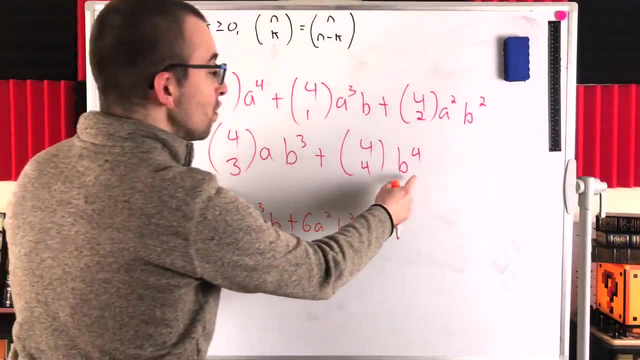 And then we're done right By the symmetric property we can. this is going to be mirrored after the six: a squared, b squared, We've got two terms over here, two terms over here. So this is the middle term and it's going to be symmetric across the middle. 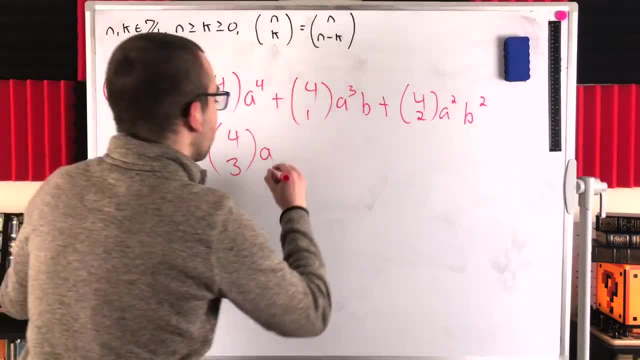 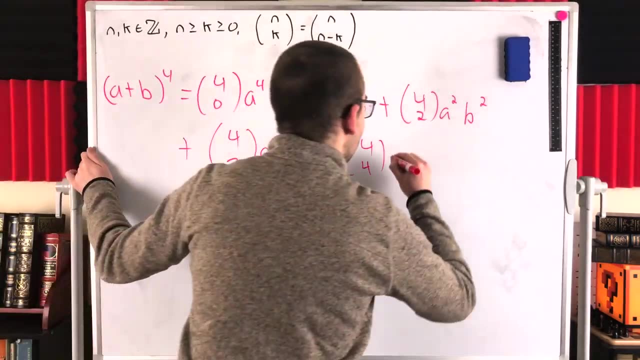 four, choose three. and then a goes down to a to the power of one, b goes up to b. cubed plus four, choose four. a goes down to a to the power of zero- that's one, we don't write it. b goes up to b to the power of four. Beautiful I could have made. 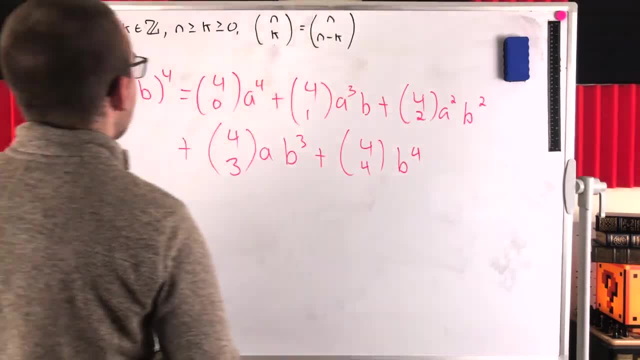 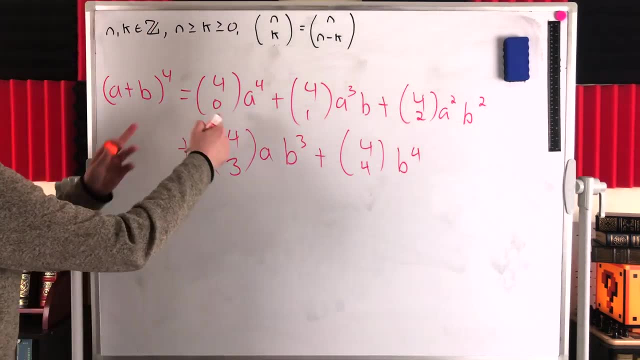 this more revealing if I had drawn everything smaller. but what are you going to do? Okay? so then say, we want to calculate the binomial coefficients here, and I've worked with these a lot. Good chance you have too. You might know some of these by heart, right? So four choose. 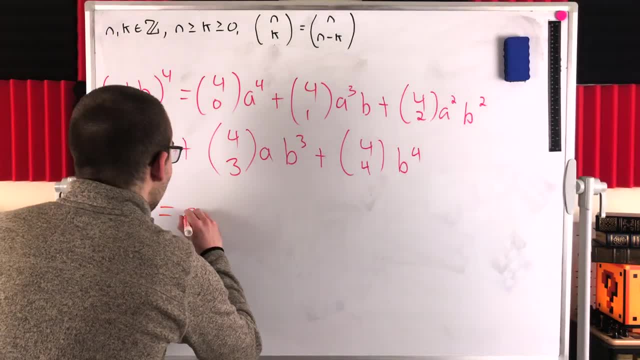 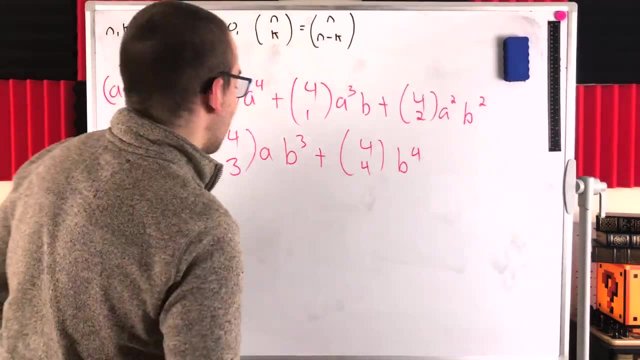 zero. What's that? Well, that's one. There's only one way. we can choose nothing. So we've got a to the power of four. Number of ways we can choose One object from four objects, that's four. So this is four, a cubed, And of course you could. 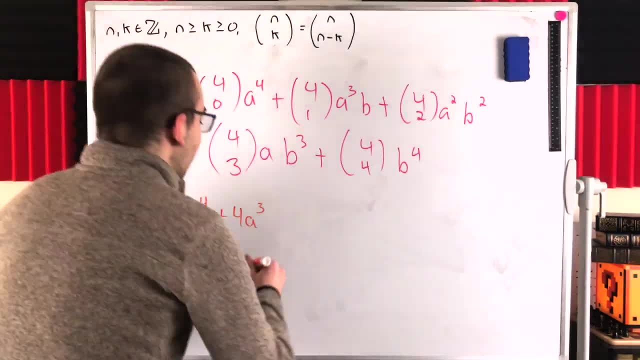 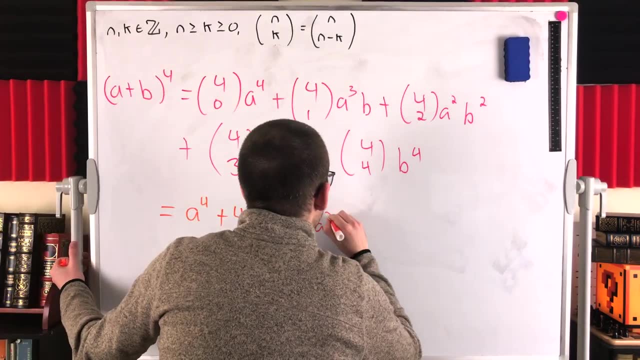 you know, use the formula here if you weren't familiar with these values. So it's four: a cubed times b, And then we've got four. choose two. that's a classic. that's six: a squared, b squared. 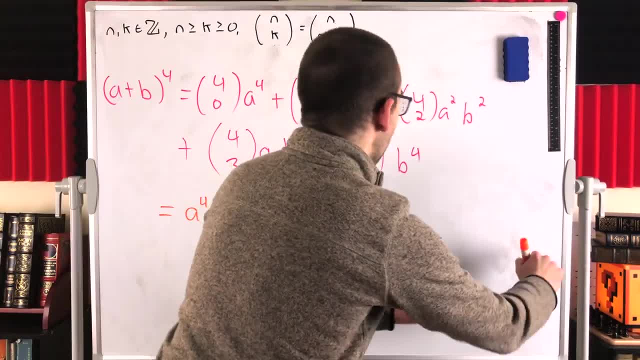 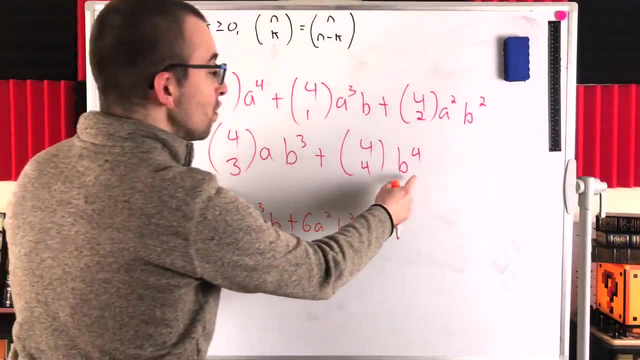 And then we're done right By the symmetric property we can. this is going to be mirrored after the six: a squared, b squared, We've got two terms over here, two terms over here. So this is the middle term and it's going to be symmetric across the middle. 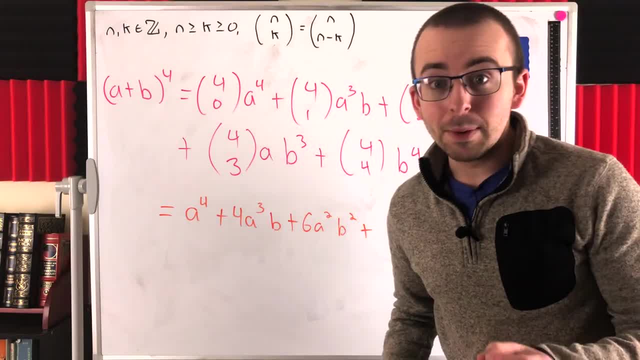 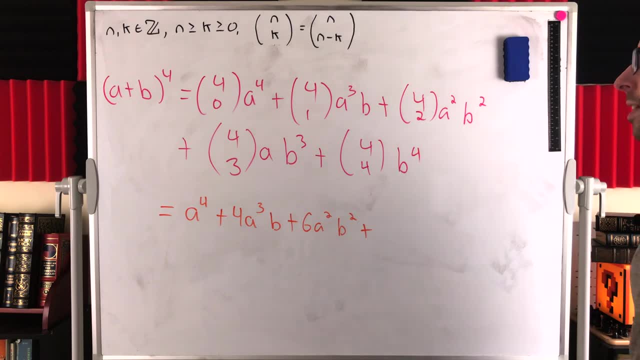 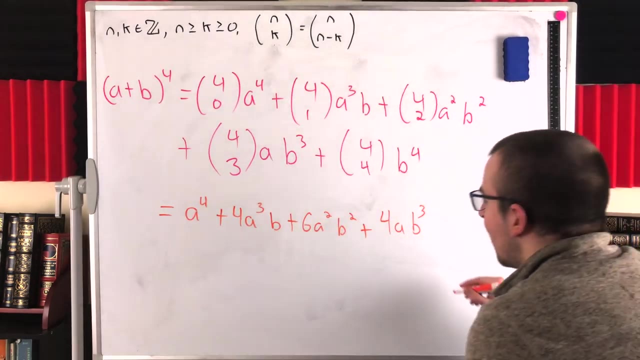 term. So what's going to be symmetric in particular are the coefficients. right, These things, because that's what's got this property. So the rest is easy peasy. It's easy pickings, right? It's four, four, a, b cubed, a, b cubed, and then plus your one times b to the power of four. 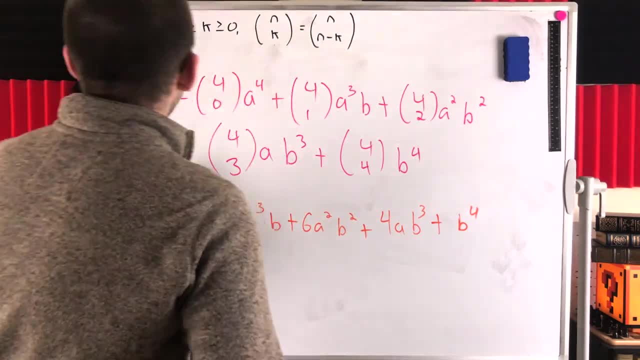 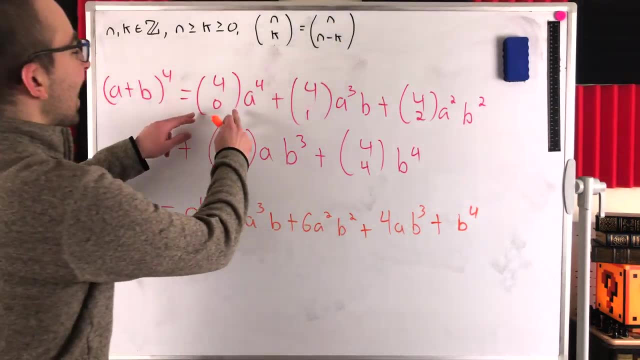 Beautiful. It doesn't save us a ton of time for a plus b to the power of four, but if it was a plus b to the power of, say, 12, then you've only got to calculate your binomial coefficients up to your middle. 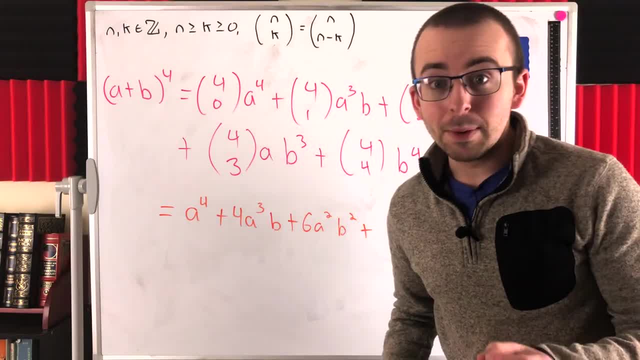 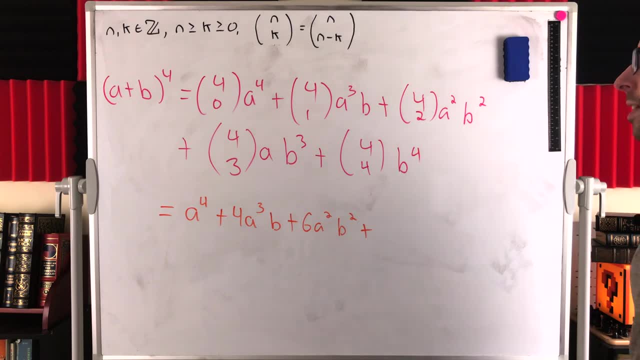 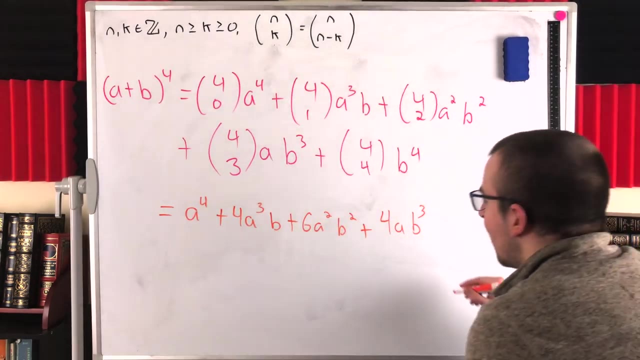 term. So what's going to be symmetric in particular are the coefficients. right, These things, because that's what's got this property. So the rest is easy peasy. It's easy pickings, right? It's four, four, a, b cubed, a, b cubed, and then plus your one times b to the power of four. 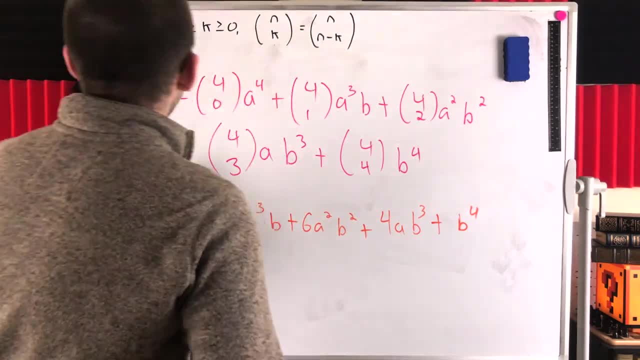 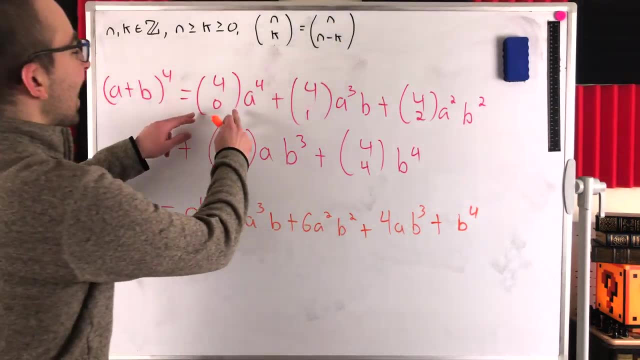 Beautiful. It doesn't save us a ton of time for a plus b to the power of four, but if it was a plus b to the power of, say, 12, then you've only got to calculate your binomial coefficients up to your middle. 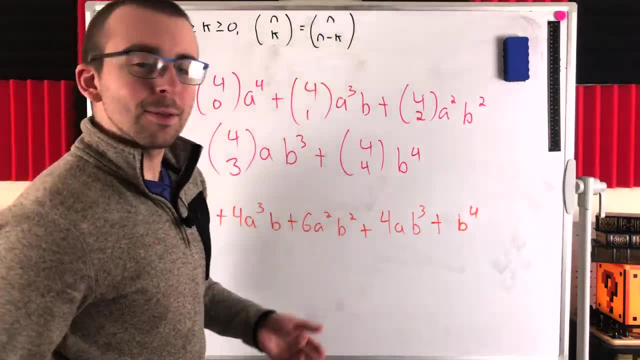 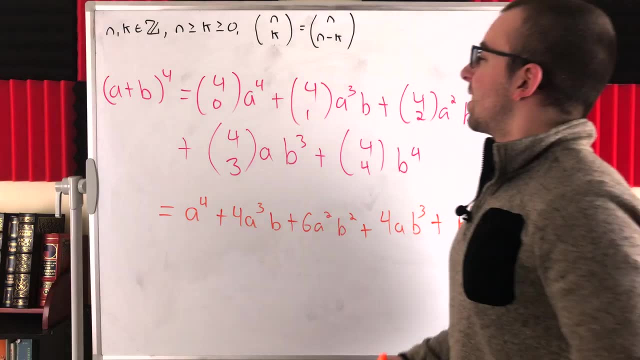 point And then, since it's symmetric, you get the rest for free because they're the same. It's just going to be a sort of mirror image. So went through that super quick because you know the primary focus of the lesson is just showing you why this is true And hopefully I've explained.